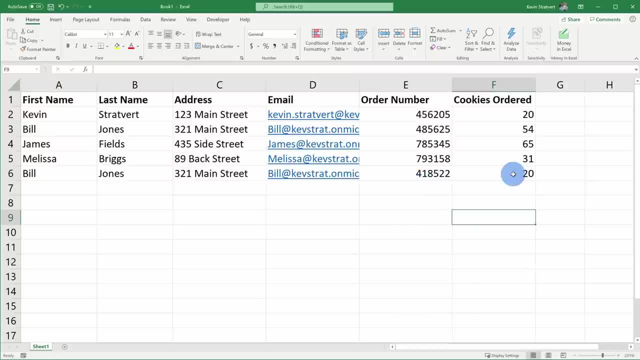 flat file. There are no relationships between this data and it's really inefficient. So here you'll see now that I've had to copy Bill's data from up here and I've had to paste it in again, So right now I'm carrying his data twice With the database. you don't have to do this. We could set up. 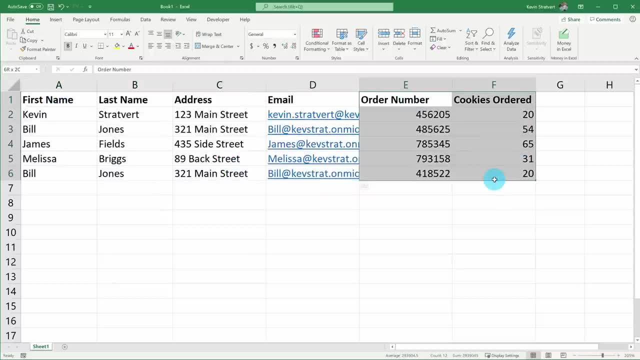 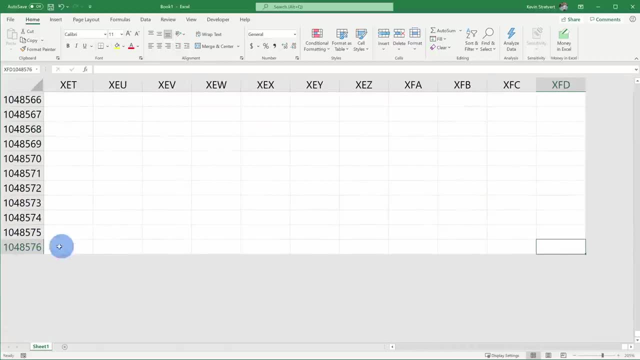 different tables for the customer information and a different table for the order information. Also, with an Excel spreadsheet, you're limited to just over one million rows of data, and so if you have more data than that, well, unfortunately Excel won't be able to handle that. 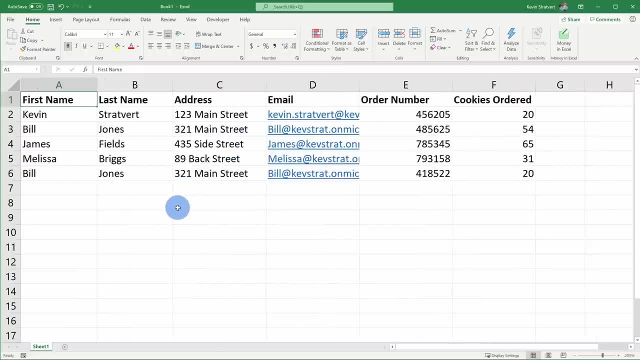 Also, if I go back to all the order information here, if I want to extract interesting insights from this data, maybe I want to write a query and I can do a little bit of that with Excel. I could filter the different columns, I could insert a pivot. 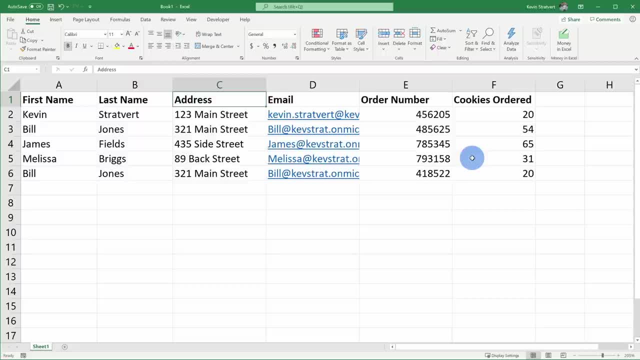 table for every single parameter and I could create a little table for every single parameter table. I could try to manipulate the data to get an interesting view, but sometimes you just need to be able to write a query and then to pull together a report and unfortunately that's not. 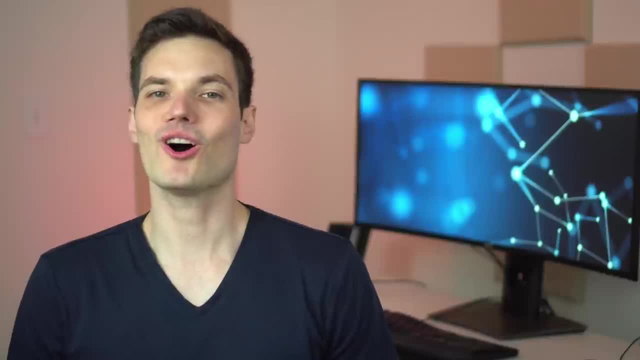 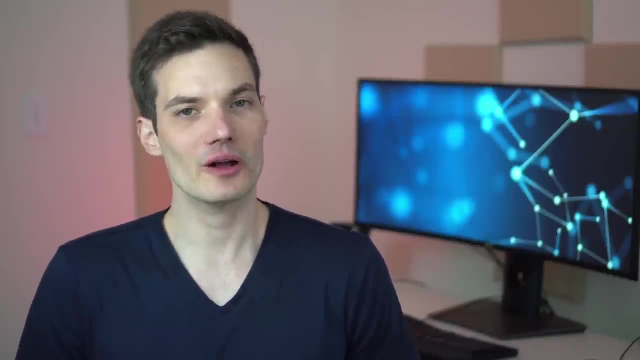 that easy with Excel, so that's where databases went out. All in all, Access is a fantastic tool for individuals or for small businesses that need to track things. However, if you're, let's say, a mid-sized company or even a large company, you'll probably start to realize some of the limitations. 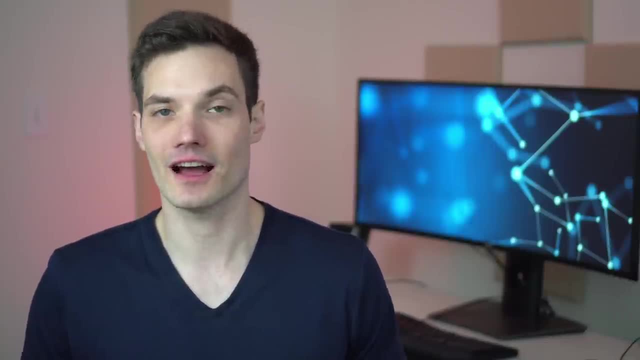 of Microsoft Access and, to be totally fair, when I worked at Microsoft, I was on some teams that used Access just as a really quick and simple database. If you're a larger company, you'll probably look at other options like Oracle, MySQL, Microsoft SQL Server, MongoDB, and the list goes. 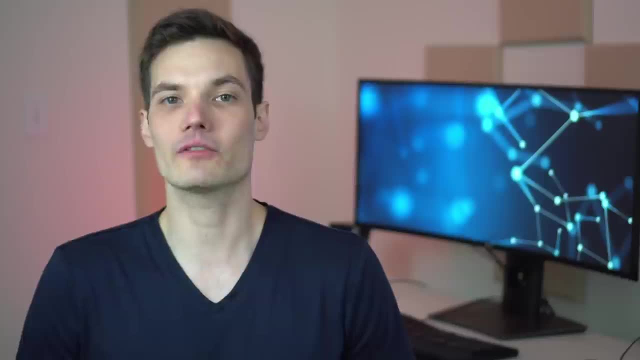 on and on of solutions that are more scalable. However, what I will say is: Microsoft Access is a fantastic tool to learn the fundamentals of database design. To learn the fundamentals of database design, you need to know what's in the database and what's not in the database. 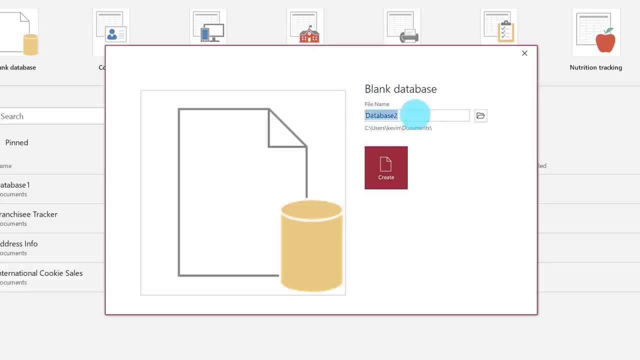 To learn the fundamentals of database design, you need to know what's in the database and what's in this tutorial. we're going to build our own database today and you're welcome to follow along. You know I've been meaning for a long time to create a database for the Kevin Cookie. 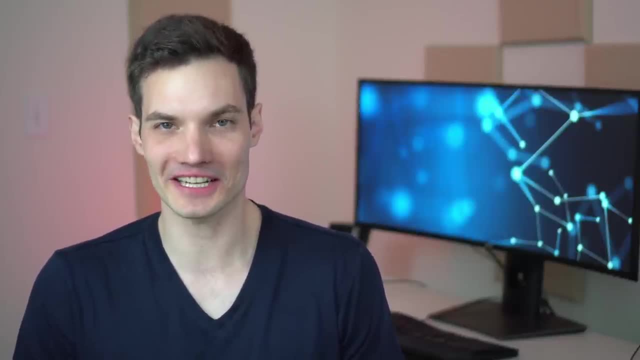 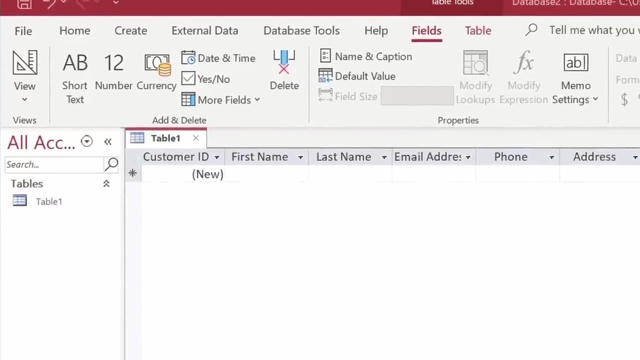 company to track our orders, and this seems like the perfect opportunity. Yes, I did figure out a way once again to incorporate the Kevin Cookie company into a video. We'll start off by creating tables, Then we'll go ahead and create an order entry form. This way, other people can come in. 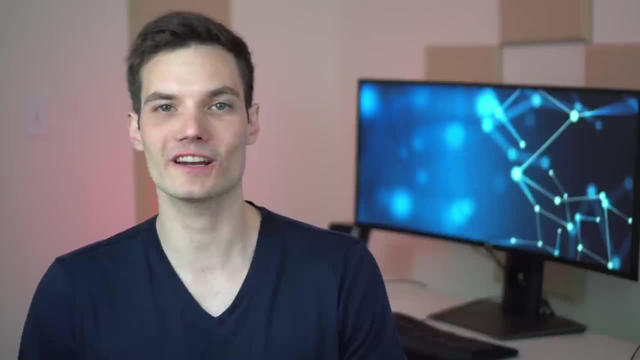 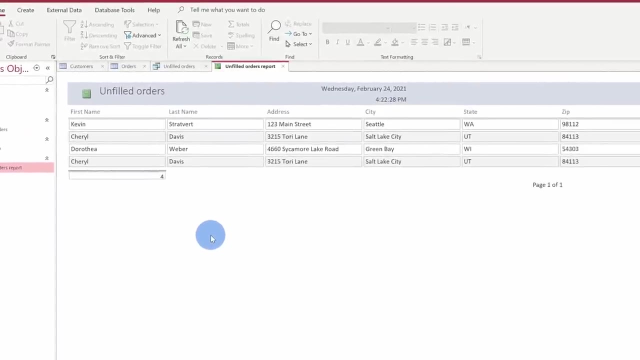 and add data to our database. Then we'll write a query so we can extract interesting insights from our data And then, at the very end, we'll create a report so we can share some of those insights with others. With all that said, by the end of this video you should have pretty good working. 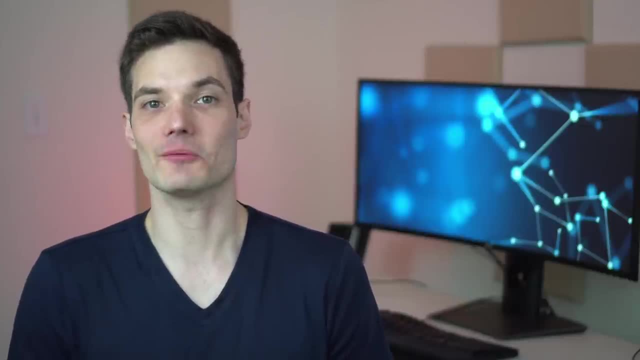 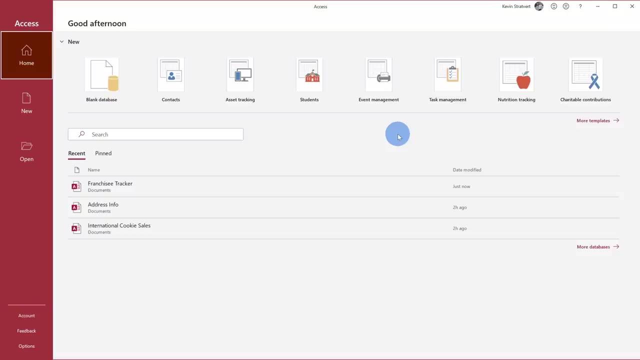 knowledge of how Microsoft Access works. All right, well, enough talk. Why don't we jump on the PC and let's start building our very first database? To get started with Microsoft Access, go ahead and launch the application and that'll drop you on the start page or right here, what's also referred to as the home view. 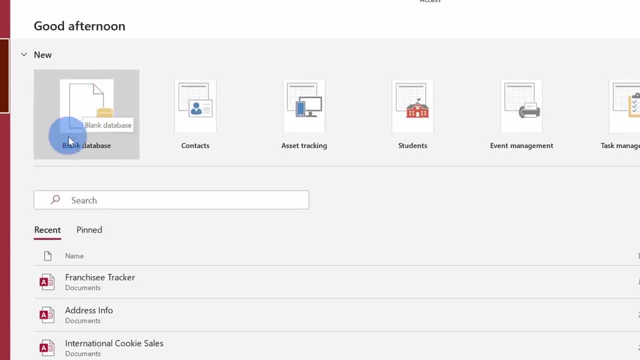 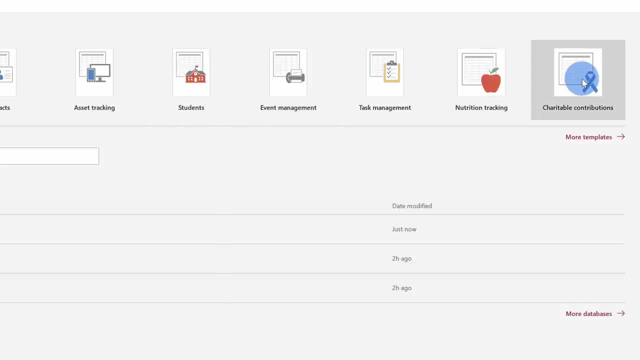 Right here at the top you can create a new database. We can start off with a blank database and in a moment we'll do that. Over on the right-hand side you also see a whole bunch of different templates. If there's a template that matches what you're trying to do, this could help. 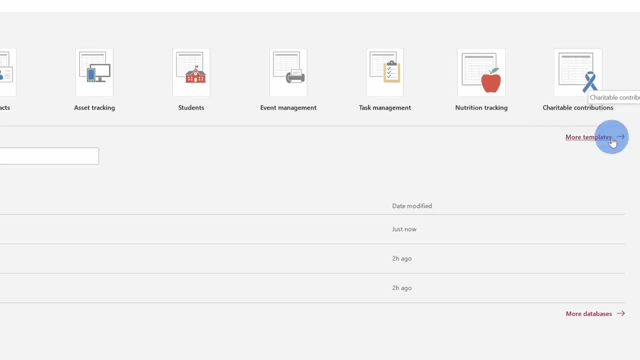 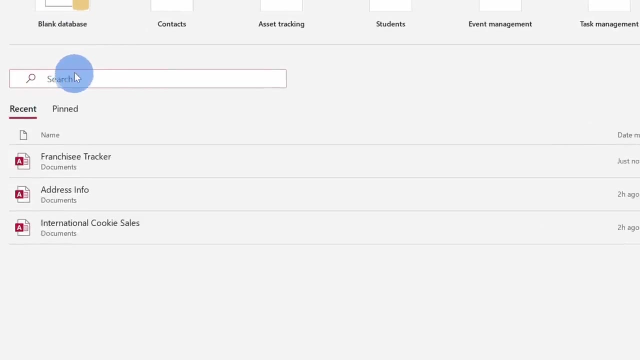 you save a little bit of time and you can go in and just tweak it. There's also a massive collection of templates that you can look at. by clicking right here Down below, you can search for different databases. You might be able to search for a couple of different databases that you might. 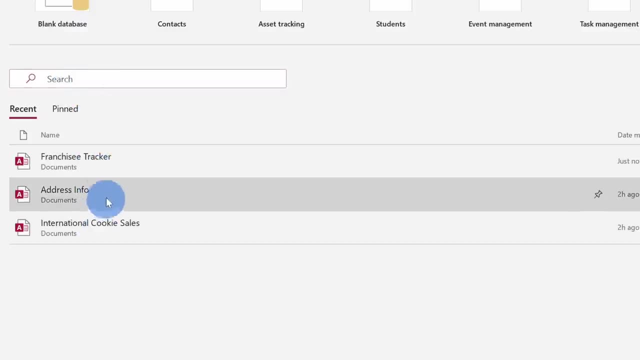 have worked on in the past, and here you can see all of your recent databases- One of my favorite features. when you hover over right here, you'll see a pin icon. When you click on this, this will add it to the pinned view. so this is just a quick way to get back to the files or the databases that 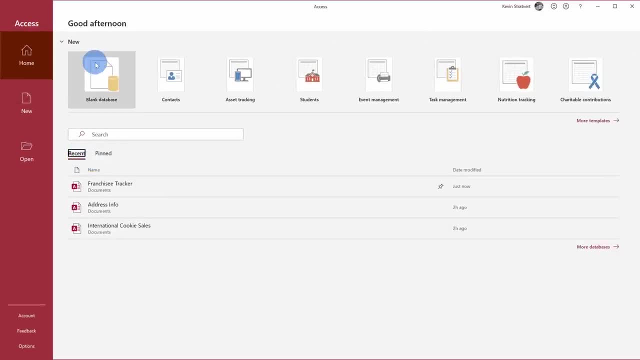 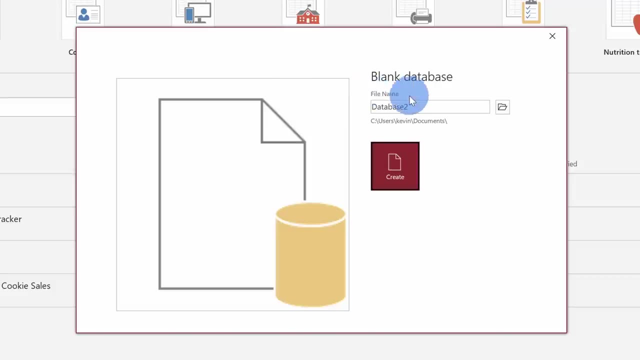 you use most often. Okay, to get started, let's go back up to blank database and let's click on this. This opens up a dialog where we can type in a file name for this database, and I'm going to call this. 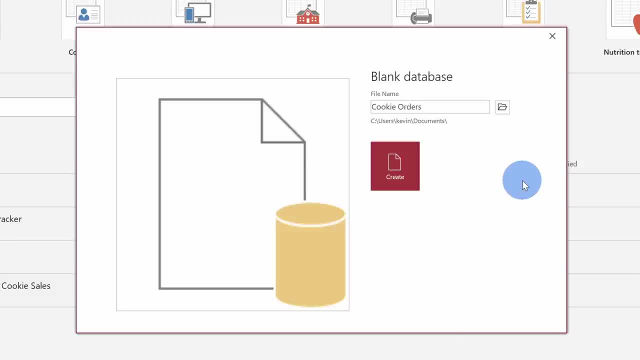 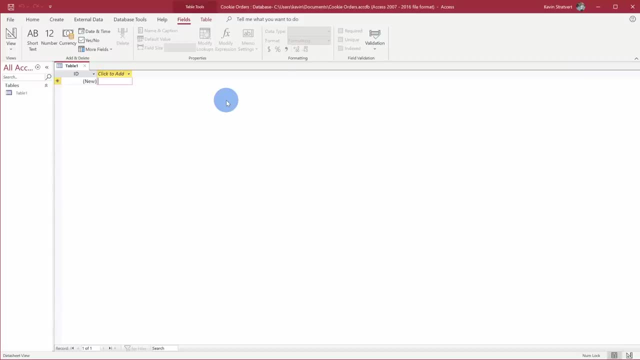 Cookie Order, And if you want to follow along, feel free to give it the same name. I'll leave it in the default location right here in Documents, and next let's click on Create. This now drops us into a new Access database, and congratulations, you've now created your first database. There's not much here. 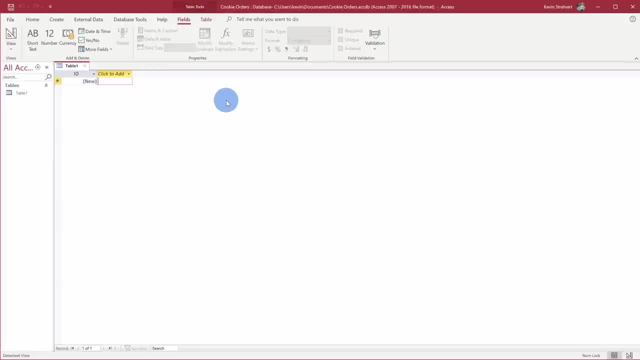 yet, but don't worry, we're going to go through step-by-step how to build this out. And before we jump in, I do want to orient you to the experience and just talk about some very, very basic database terminology. Over on the left-hand side we can see that Access created. 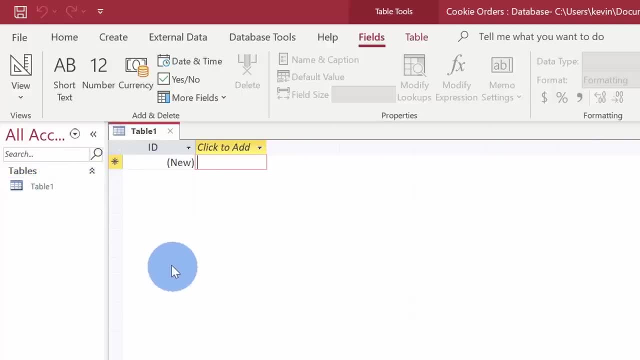 Table 1, and we're going to start building out Table 1 first And, like I said, I want to track customers and orders for the Kevin Cookie Company, so we'll use Table 1 to track the customer information. So we're going to keep that separate from the order information. Also over here on the 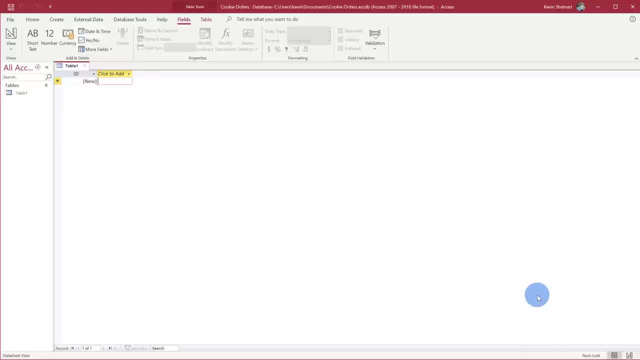 right. if you've ever used Microsoft Excel before, this probably looks familiar. We have all of these different cells. The terminology here is a little bit different. In Excel we refer to these as columns, and we refer to these as columns. 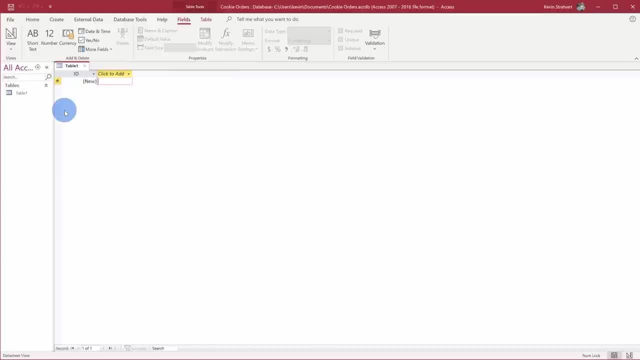 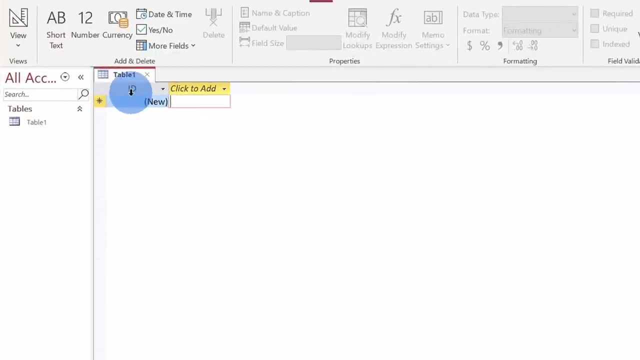 We refer to these as rows. In Access it's a little bit different. We refer to a column as a field and then a row is referred to as a record. So we're going to be adding records to our database. Let's get started now by adding some fields to this table Now up here. the first field is: 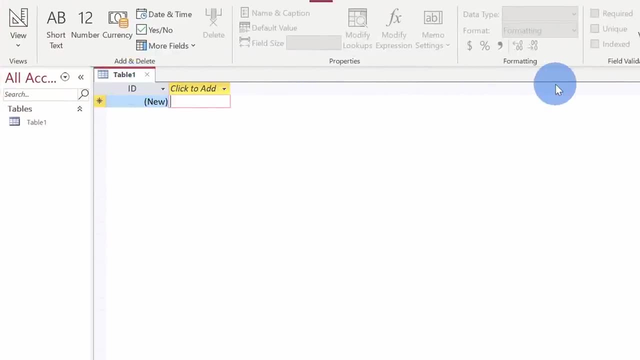 referred to as ID and once again I want to use this table to track all of our customer information. ID on its own isn't that descriptive. I want to update it to be customer ID. So to update the name you can simply double click on the field and then here I can type in my own value. 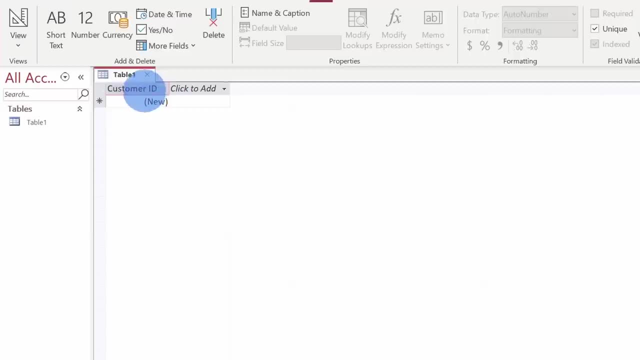 I'll type in customer ID and that looks good. now, Once I'm done typing that in, hit the tab key and that'll bring you over to the next field and here, first off, you need to choose the data type: The. 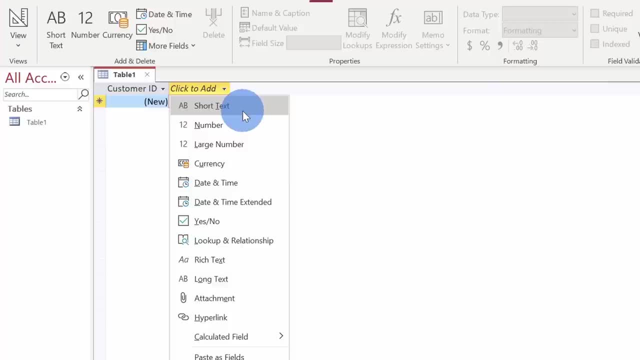 data type defines what type of data you're going to insert in For this. I wanted to track customer information, So this is going to be things like the customer's name, the first name, the last name, the email address, the phone number and the number of customers that are going to be added to the table. 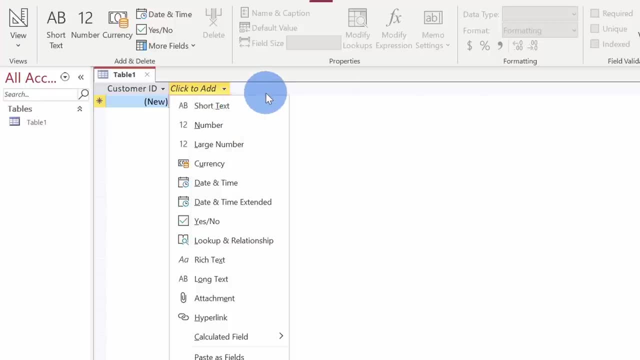 And all of those pieces of information, or all of those fields, will simply be the short text data type. However, later on, when we get to the order sheet, we're going to add numbers, and so we'll select a different data type. As you're entering data, feel free to look through all the data types. 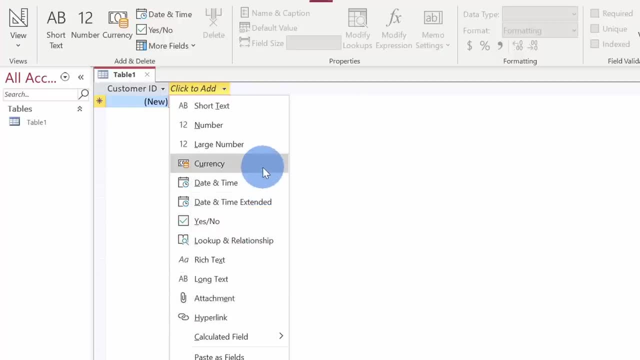 to see if one of these best matches the data that you want to enter For the first field. I want this to be the first name, so I'll select short text. Now it's called short text, but it allows up to 255 characters, which is actually a pretty good. 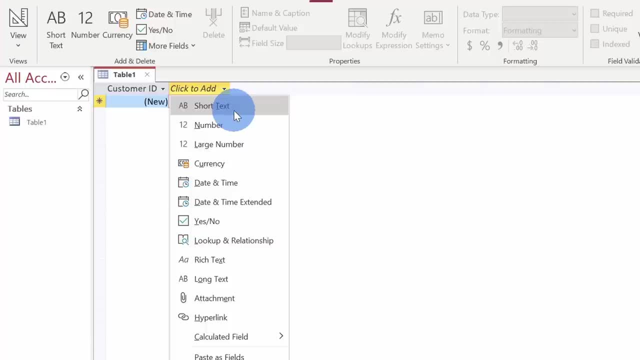 length, So it'll capture all of the different fields that we want to insert into this table. If you want long text that allows it to go much, much longer, but once again, short text should be sufficient. I'll select this Once I select that data type. now I can type in the name for: 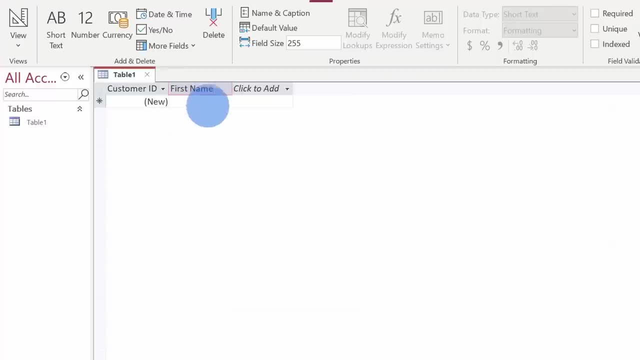 the field. I'm going to call this first name. Once I finish typing that in, I'll hit tab and here I can select the data type for my next column And for this one. this is going to be the last name And I'll go through and add all of the different fields for the customer tracking table. 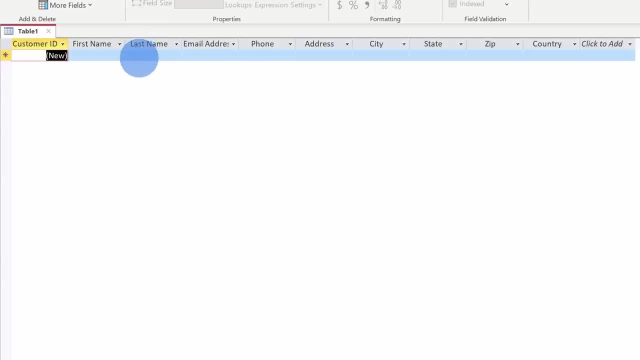 I've now added all of the different fields to this table and if you're following along, feel free to pause this video and you can then enter in all of these different fields. The data type for all of these is short text. At the very end I want to add one additional field. 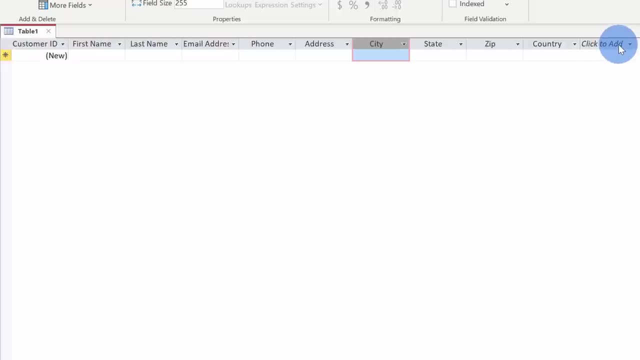 and this one's going to be notes. So let's say, maybe a salesperson for the Kevin Cookie company comes in, they add a customer and maybe you want to include things like the customer's kids' names. There's nothing like remembering the customer kids' names to close a deal. Or maybe you want to 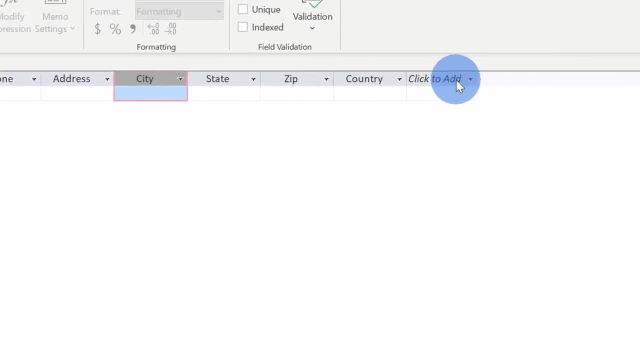 include other information like the name of the customer, or maybe you want to include other information like the customer's kids' names to close a deal, Or maybe you want to include other information like the customer's birthday, all that type of stuff, And this might be a little. 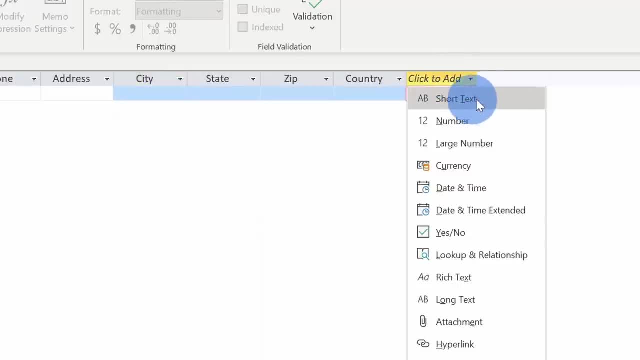 bit longer than short text, So here I'll click over here and instead of going with short text, I'll go with long text, And for this field, I'll call it notes. This should now include all of the different fields that we want to include as part of this customer table. 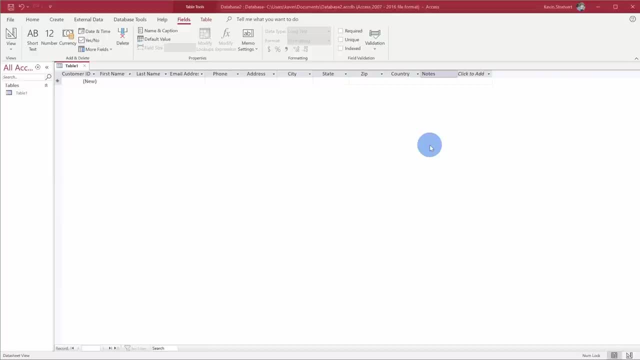 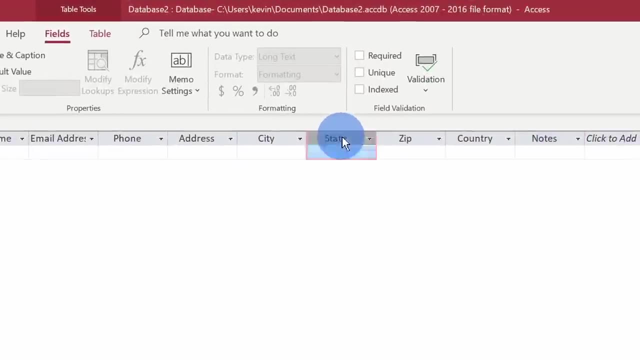 Now that we've entered in all of the different fields, I want to show you how you can go back and make edits to these. So let's say, you enter something in but maybe you screwed something up or you want to change the text Right here. I can click on one of these field headers and you can. 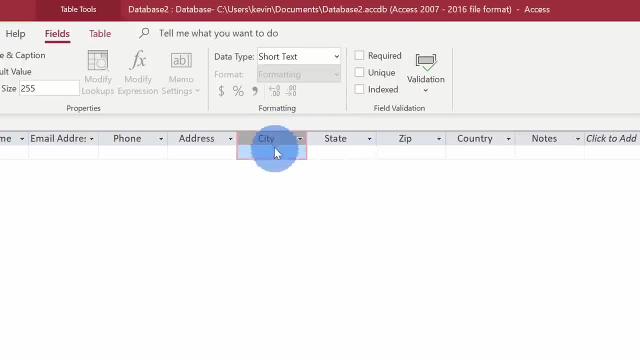 very quickly update the text. Also, when I click on one of these field headers right up here, that opens up the fields ribbon And right here I can always go back and modify the data type. So just because you choose a data type doesn't mean you're locked in on it. Right down below I can: 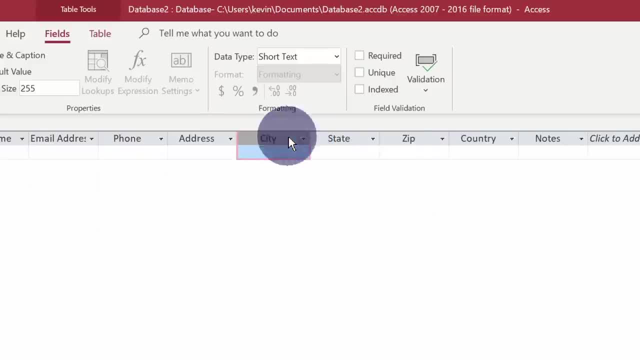 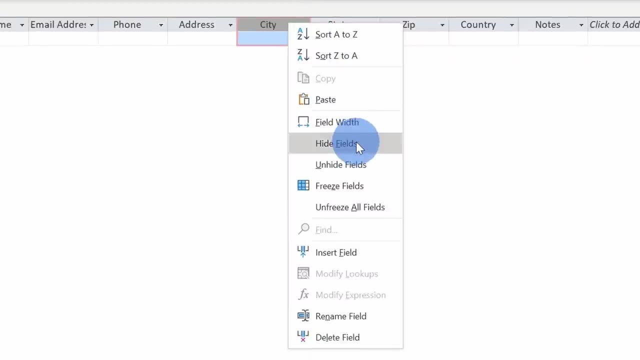 also adjust the width of these different fields. And here, if I right click on one of these field headers, it opens up a context menu where I can do all sorts of things. For example, I can hide fields. I could also unhide fields Here. you could freeze fields, if you've ever done that in Excel. 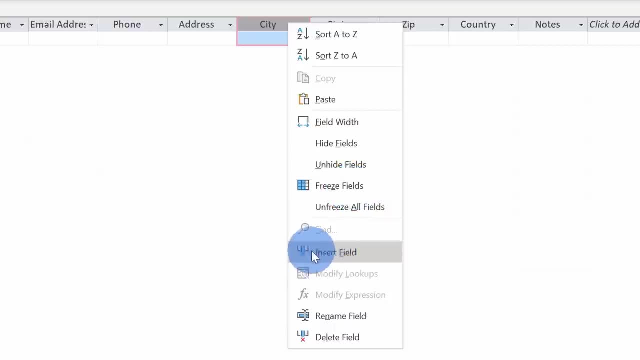 before. It's the same exact concept And right down here I could insert a field. Let's say I want to insert something between email address and phone. I can do that. I could also rename here again and I can delete fields. So all types of different actions I can take to make sure that the 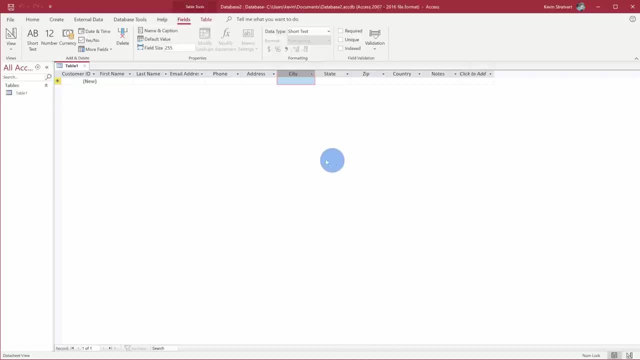 table has the structure that I want it to have. Now that we've gone through and we've created all of our different fields, I want to show you a quick way where you can look at your fields and also modify the different data types. Down here in the bottom right hand corner, you can enter. what's called the design view And you can see here. you can go ahead and create a new field And you can also modify the different data types. Down here in the bottom right hand corner, you can go ahead and create a new field And you can also modify the different data types. And when I click, 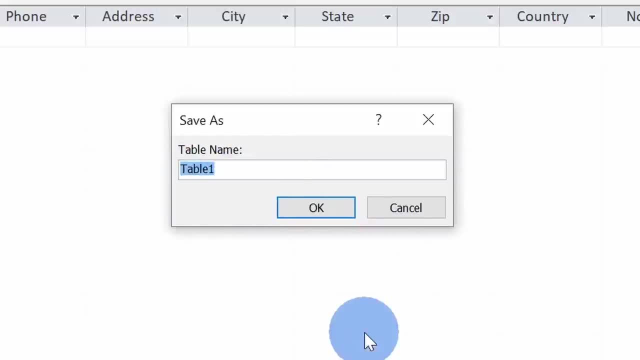 on that. first, I have to name my table. Right now it's table one, but I want it to be more descriptive. Once again, this is tracking customer information, So I'll call this table customers. Once you've finished typing in the name, click on OK. This now drops me into the design view. 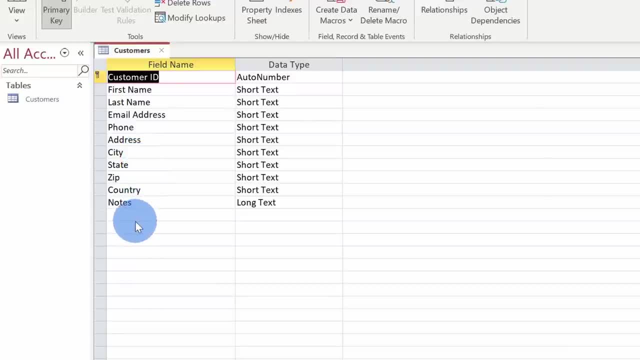 And here again I can see all of the different field names. You can also add field names here. This is a pretty quick way to add additional fields. Also over on the right hand side here you can quickly verify what the data type is for each one of your fields. 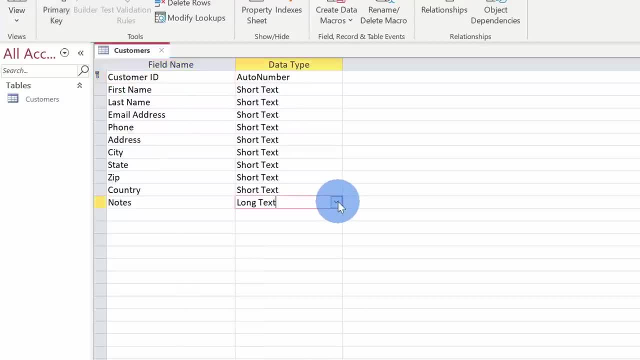 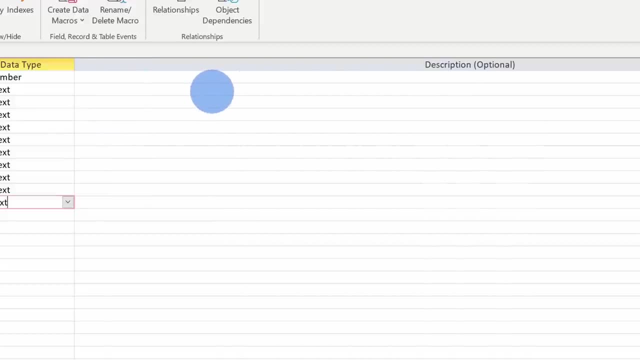 And here too you can click on it and you can change the data type very easily Over on the right hand side. let's say, maybe your field name's not really that descriptive. you can also add a description with some additional details. Let's jump back into the data sheet view To do that, right down in the bottom right. 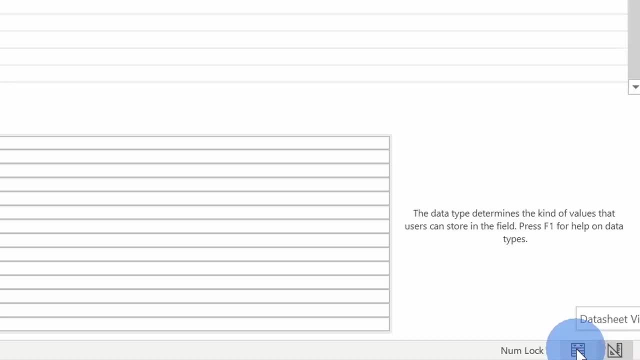 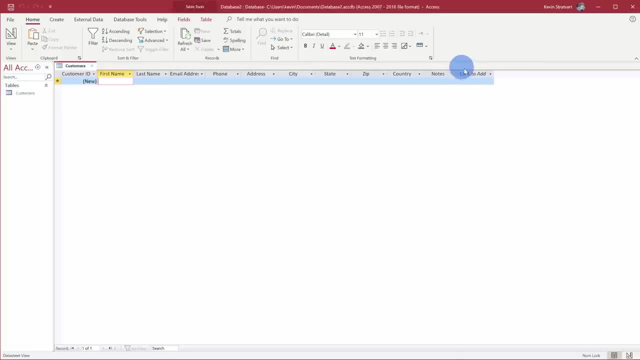 hand corner. again, we can toggle back and forth between these different views. I'll click into the data sheet view. This drops us back into the data sheet view and we're ready to start adding some records. Right now we have all of the fields in place and I want to add the first customer. 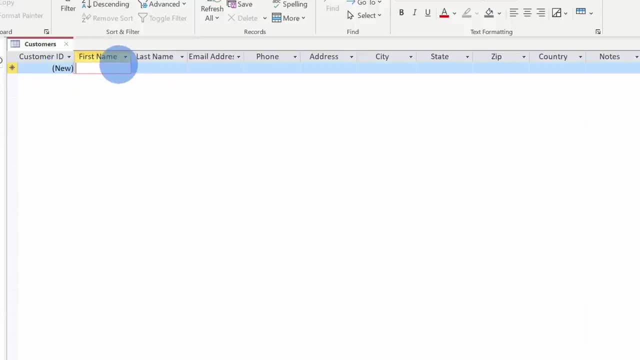 and the first customer is me. I'm probably one of the best customers. Anytime we finish a batch of cookies, I end up eating a lot of them. So right here I'll go in and fill out my details. Feel free to do the same for yourself. Here I'll type in my first name, I'll go over and I'll type in. 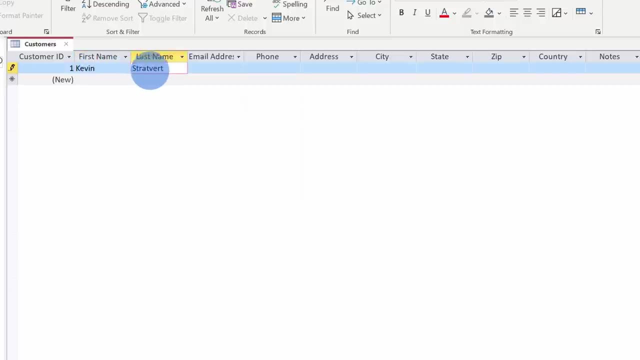 my last name, One thing to call out as I start typing in information here. you'll see that it automatically assigned an ID. So every time you go through and you add a new record, it'll automatically get an ID assigned to it. As a quick note on that: 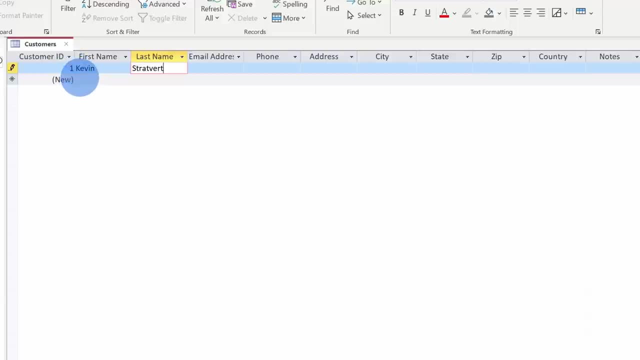 you'll notice that every single customer that we add on this ID- this is also what's referred to as the primary key. And what is a primary key? Well, this is a unique identifier. So, basically, every single customer record that we add to this table will have its own unique identifier. So no, 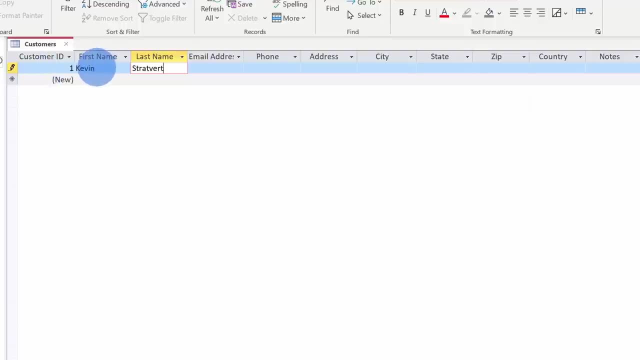 other customer will have the same ID as me And, of course, I'm the number one customer. I probably eat the most cookies, so it's really fitting that I have the number one. We're also going to use this ID And don't worry if that sounds complicated- I'll show you exactly how we go about doing that. 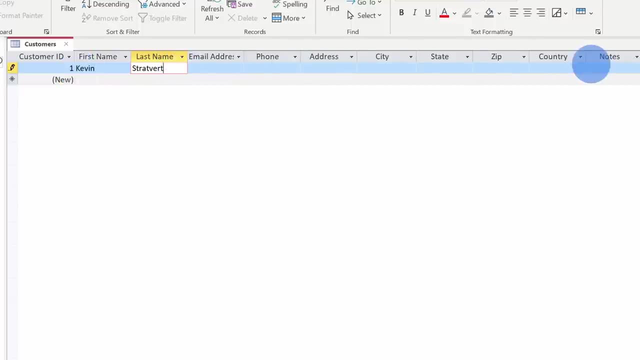 In the meantime, let's go through and fill out the details of the first customer. Once you enter in the first customer, hit the enter key and that'll bring you down to the next record, And now you can go through and add some additional customers Now, just for purposes of this demonstration. 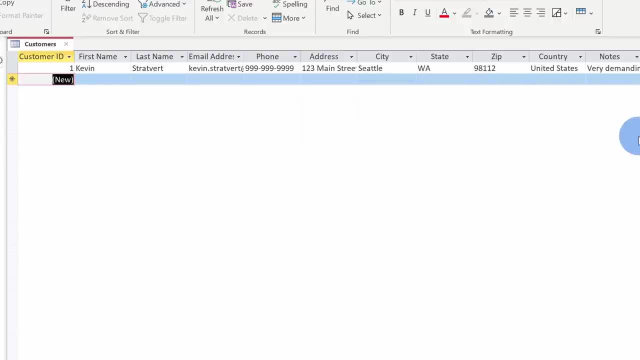 I want to go through and maybe add about four or five different customers, just so. we have some examples in the data. Feel free to do the same and make up some customer information. I've now entered in a bunch of sample customer information. If you don't want to type in customer information, 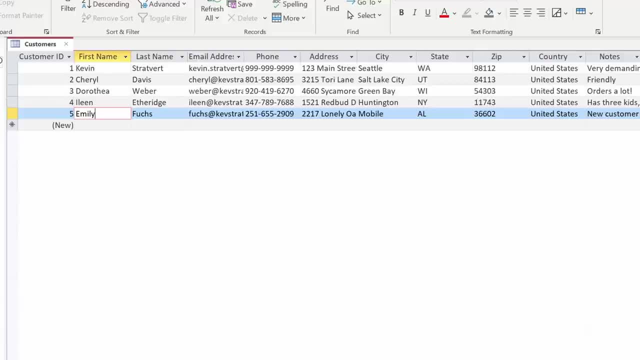 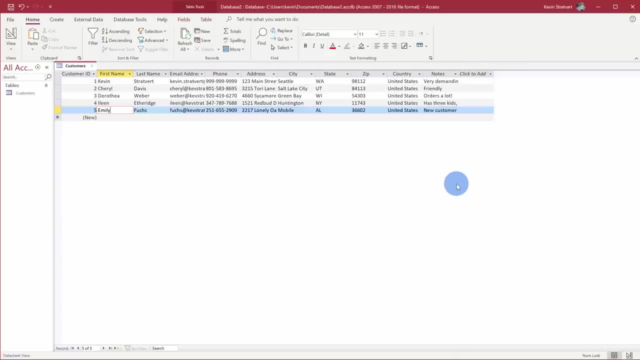 but you still want to follow along. I've included a link to this database in the description. This will allow you to access this database. We've now finished all the customer information and I now want to add one more table with all of the order information. To add another table. 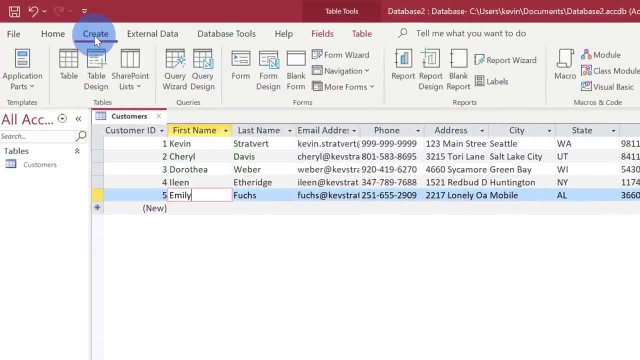 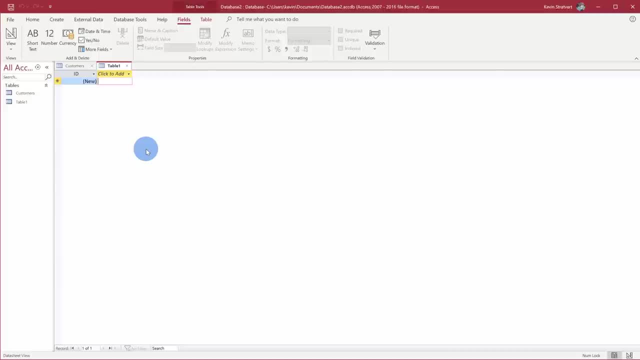 let's go back up to the top ribbon and let's click on create. Right over here we can create a new table. I'll click on the one that says table. This drops us into a new table and it's called table And, just like before, we need to build this out Right up here. 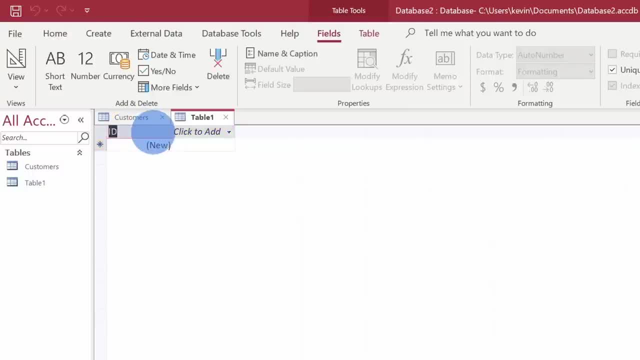 the first field is called ID, and I want this to be more descriptive. I'll double click on this, just like we did before, and this time I'll call it order ID For the next field. I want to tie this back to the customer's table. Once again, this is one of the big benefits of databases. 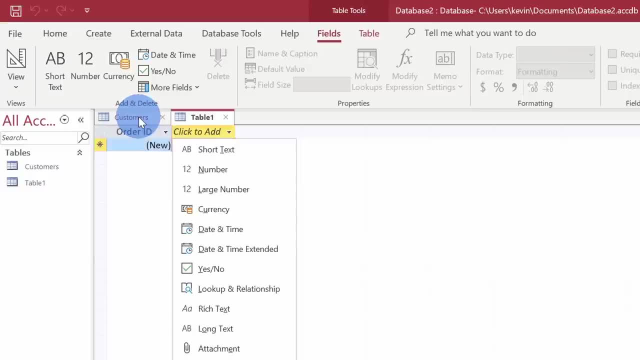 You can relate information, So you can connect one table to another table. So here I'll click on tab and for this field I want it to be a number data type. For this one I'm going to type in a field name. For this one I'm going to type in customer ID. 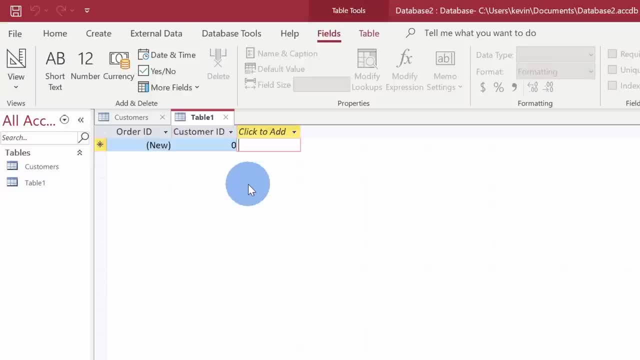 We're going to connect based on that primary key from the previous table. I want to add a few more fields. For this one I want to include the order date, and a date is a date and time. I'll select that as the data type and here I'll type in order date. I'll add another field for cookies: ordered. 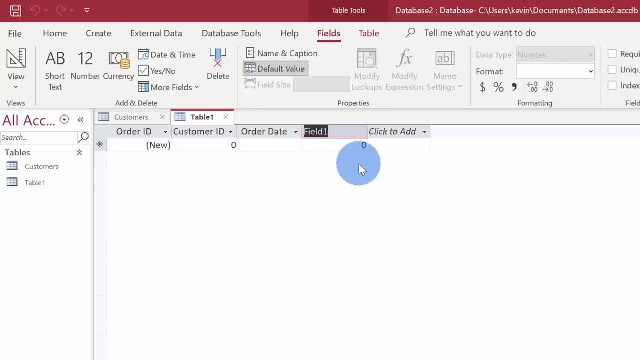 and this is going to be a number data type. Here. I'll call it cookies ordered. I'll add another field for the revenue Here. I'll click over here and this is going to be a currency type. Next I'll type in revenue. I'll add one more field called order filled. 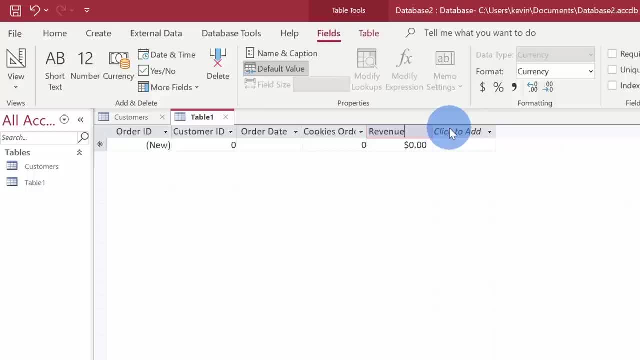 This is basically so our warehouse staff can go in and indicate whether the order has been fulfilled or if it's unfulfilled and they still have to package it and ship it. Here I'll click on this field and right down here there's the option for yes- no. So if they say yes, 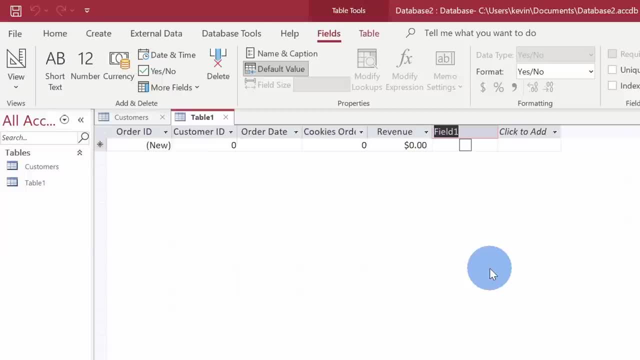 it's already been shipped. If not, it hasn't, and I'll call this field order filled. Lastly, I want to add one more field. However, this one is going to be a little bit different. This is going to contain the revenue per cookie, and we have all of the information stored within. 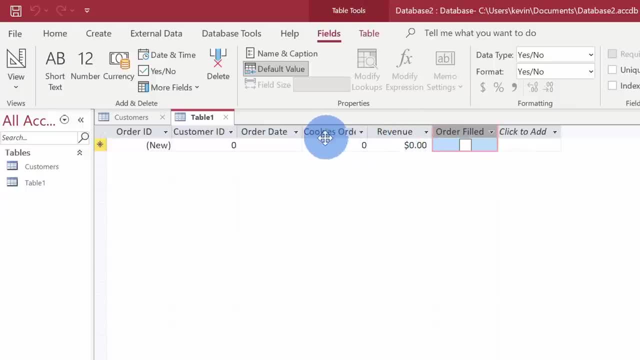 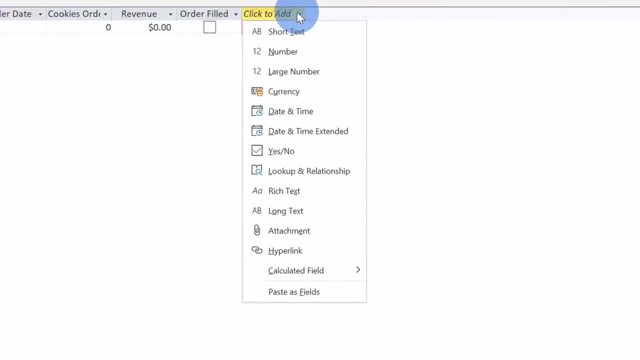 here to be able to calculate that. Here I'll have the revenue and I'll also have the number of cookies ordered. So right here let's click on this drop down where we can select the data type, and this is going to be a calculated field. We'll see in a moment what this does, Right down here. 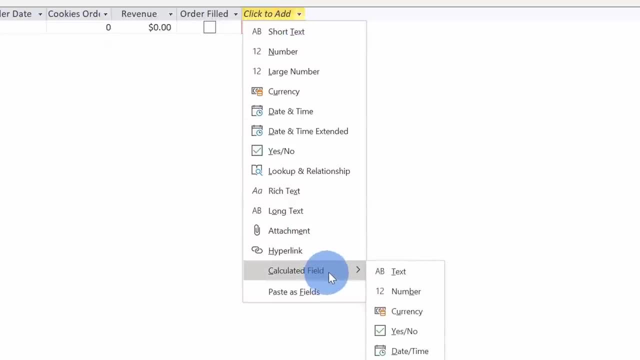 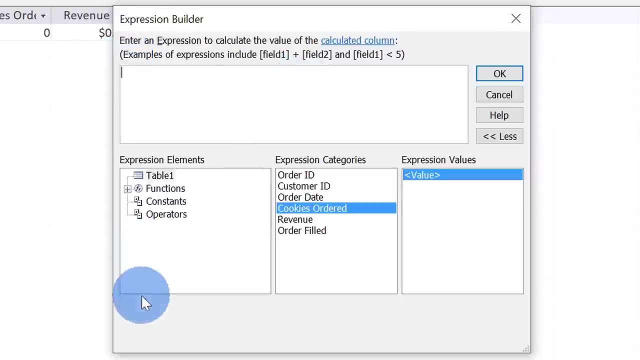 let's go down to calculated field and revenue per cookie. That's going to be a number, so let's select the number data type. This opens up an expression builder in and you can build all types of different expressions. One way to think of it is: 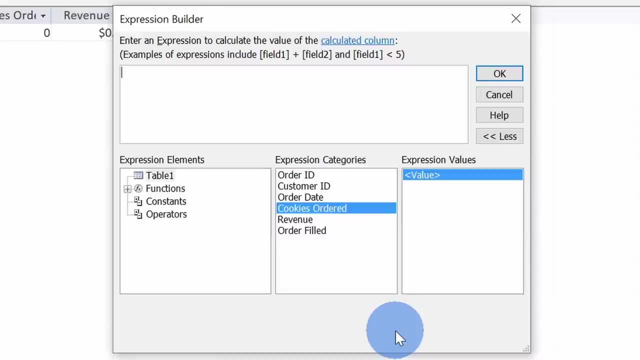 it's kind of like entering in a formula. Now, once again I want to calculate the revenue per cookie. So down here I see some of the expression categories. I'll take the revenue and when I double click on that you see it inserts revenue here and I want to divide by the. 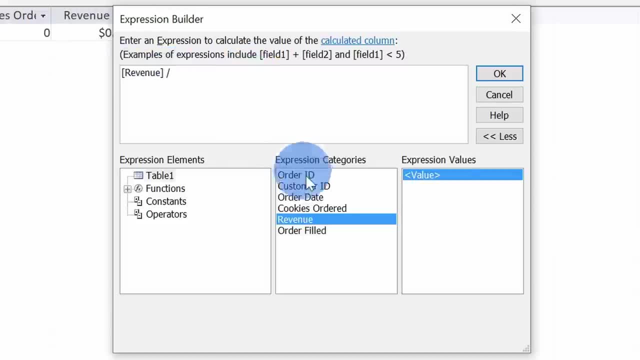 cookies ordered. So I'll enter the divide sign and then right down here I'll click on cookies ordered. So I'm gonna take the revenue divided by the cookies ordered. That looks good. Next let's click on okay. This drops me back to the tab where we can see all of the applications, and we've 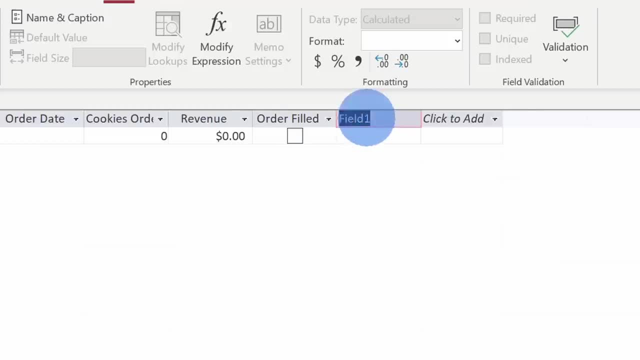 got all of the applications added to the dashboard. Now, let's go ahead and broadcast this one. Now let's. This drops me back into the table view, and now I can type in a name for the field. For this one, I'll type in revenue per cookie. 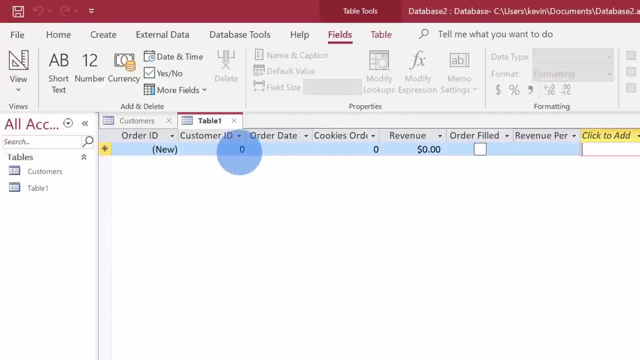 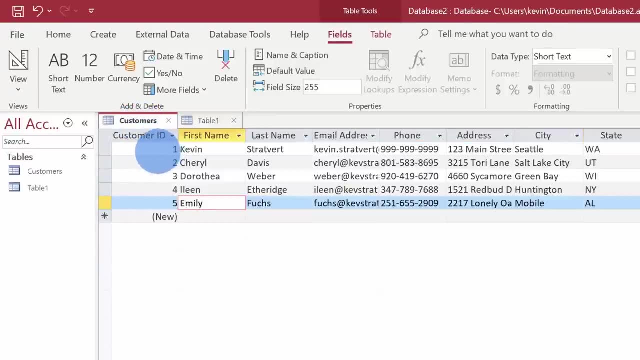 I can now fill in some order details. So over here for the first customer, this will be Kevin, who orders some cookies. Now, if you remember, back on the customers table, customer ID one is for Kevin. So right back here in my order table I'll type in customer ID number one. 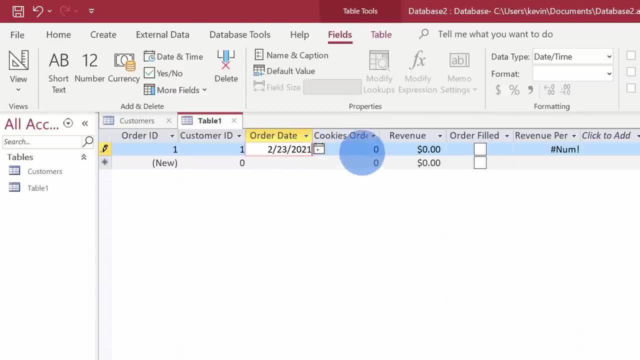 Right here I'll enter in the order date. I entered in an order date and here I can type in cookies ordered Now. if you know Kevin as a customer, he really loves cookies. So we're going to put down an order for 50 cookies. 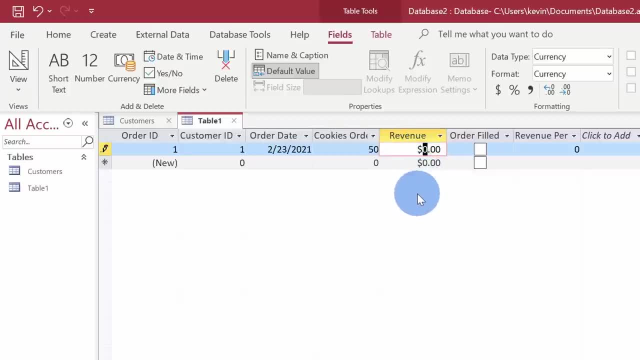 And these were some pretty premium cookies. They're about $2 per cookie, So I'll enter revenue of $100.. Now that I have that entered in, one thing you'll see is it automatically calculates the revenue per cookie Right over here. the order hasn't been filled yet. 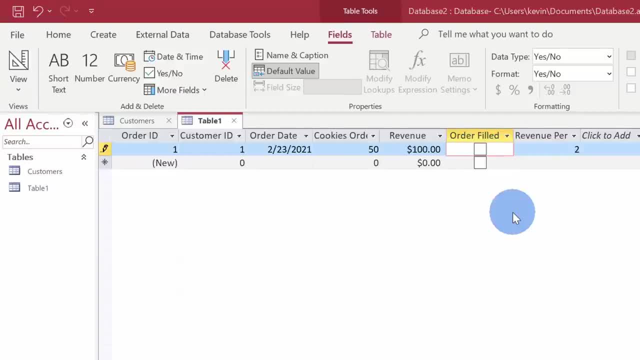 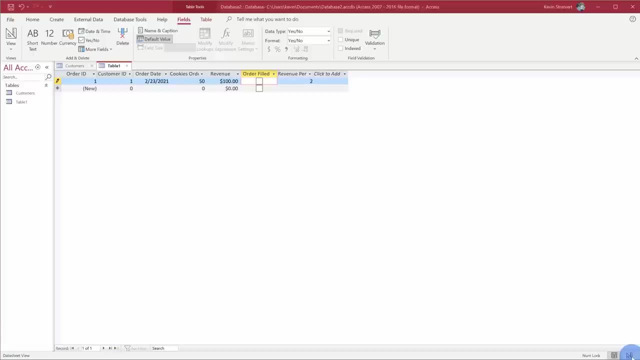 So I'll leave that checkbox unchecked Now that we finished filling out the basic structure of this table once again, if we want to rename it, we can go down here and click into the design view and then we'll be Able to rename this. 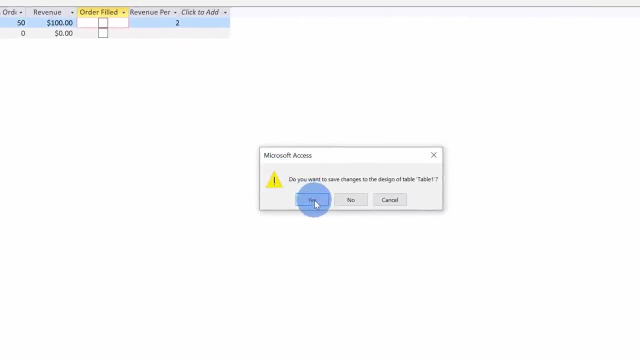 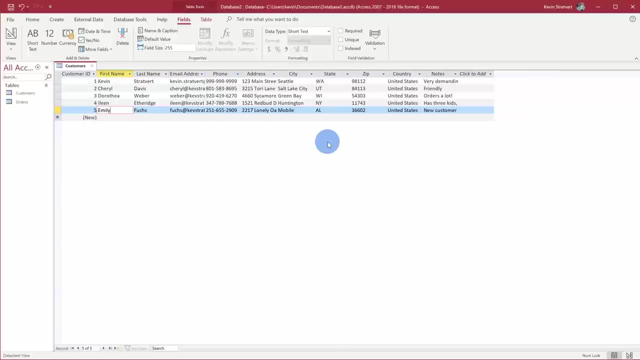 Alternatively, I can also close this table and it'll ask me if I want to save it. I'll click on yes And here I can now give it a name. I'll call this table orders. I've now finished saving my orders table and over on the left-hand side you'll see. 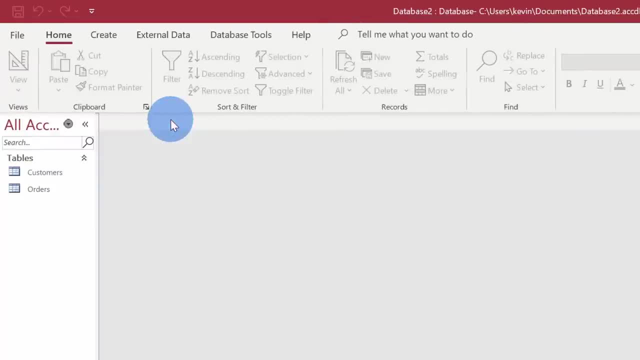 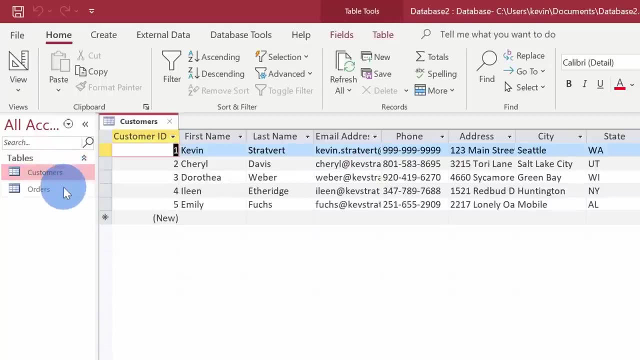 that I have two tables. Now I can go up here and I can close the customer's table, and now all of my tables are gone. but don't worry, We can easily get them back over. on the left-hand side I can click on customers and I can click on orders, and that brings those tables back. 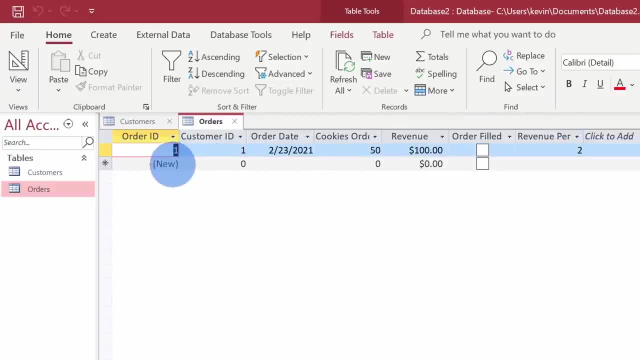 into view. I now want to go through and add Some additional sample orders, So I'll go through and maybe type in five or six different orders. I've now gone through and I filled out a whole bunch of sample data. Now, one of the great things about creating a database here: you'll see with the customer. 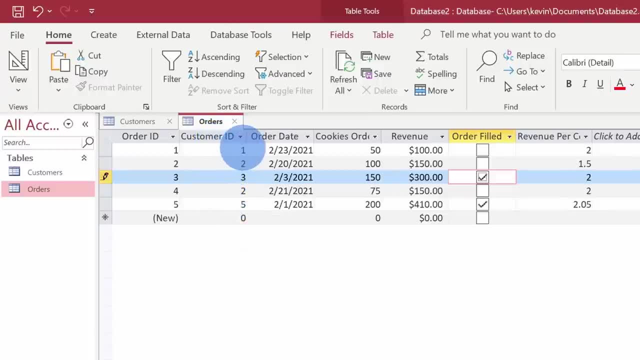 ID. I don't have to repeat the customer information. I simply have to reference that ID And then, for this order, I can fetch all of the customer information. However, first off I have to connect this customer ID to the customer table over here. 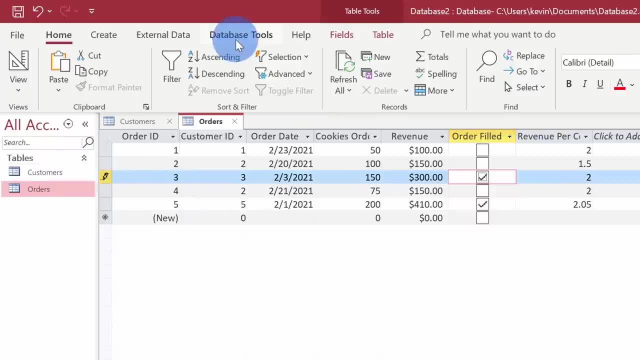 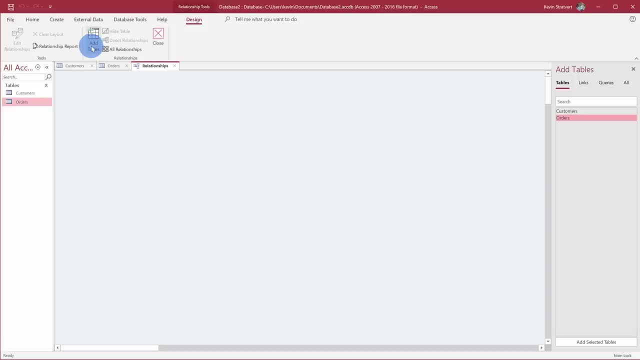 How do we do that? Well, up At the top, let's go up to database tools on the ribbon. Once we click on that, there's an option for relationships. Let's click on this. within relationships, I can define how different tables relate to one another. 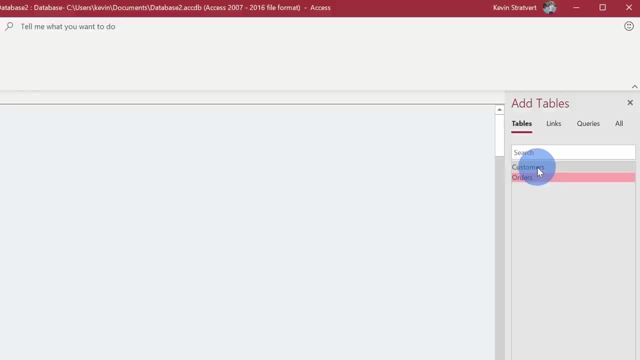 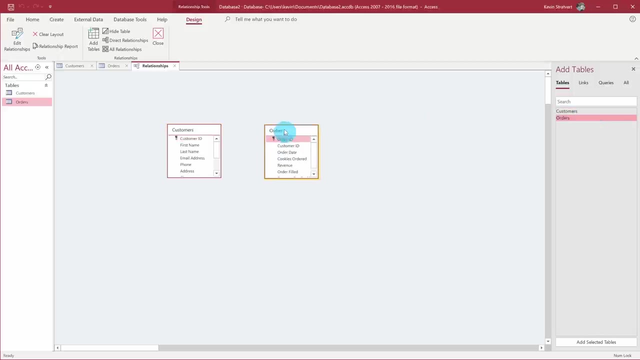 And over on the right-hand side I see all of my tables. I have two tables. I'll click on customers and I'll pull that into this view. Next, let's go over to orders. click on that and pull that over as well. 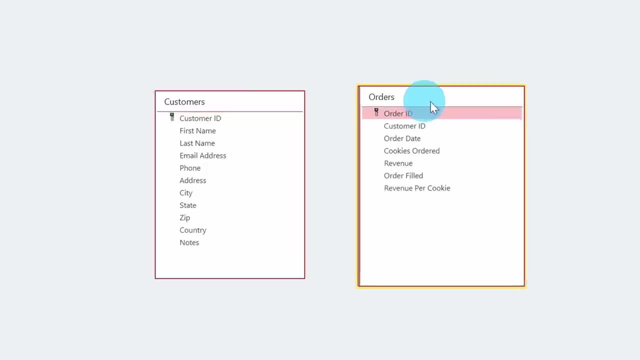 So here now I see my two tables and you can see all of the fields in those two different tables. right up here You can see a key icon and that indicates what the primary key is in that table. Now here I have the customer ID in my orders table and I also have the customer ID in 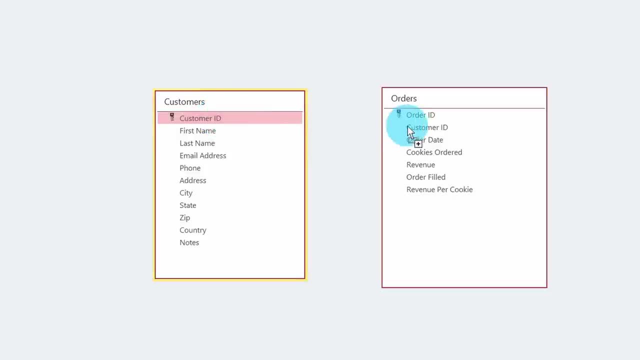 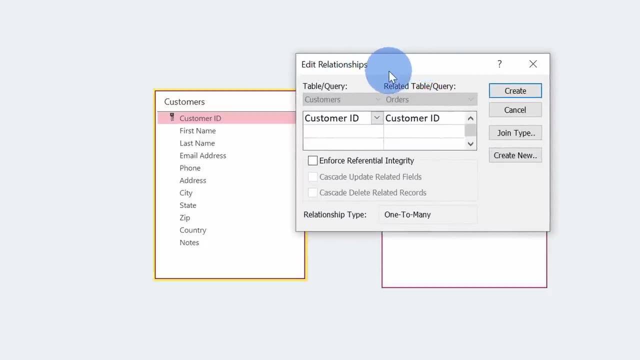 my customers table. Now I can simply click on the customer ID and I'll drag that over to the customer ID over in the orders table. That opens up a prompt where I can edit the relationship. So here I'm saying that this value or this field in the customer table is the same as this: 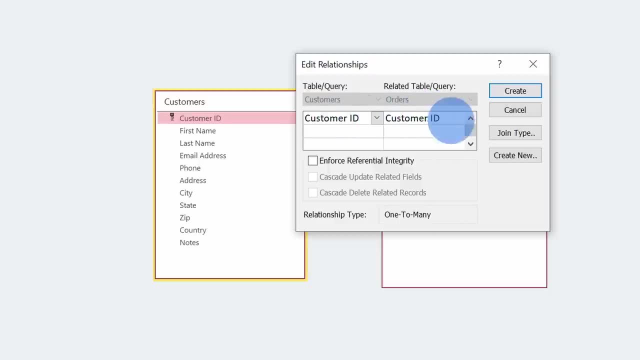 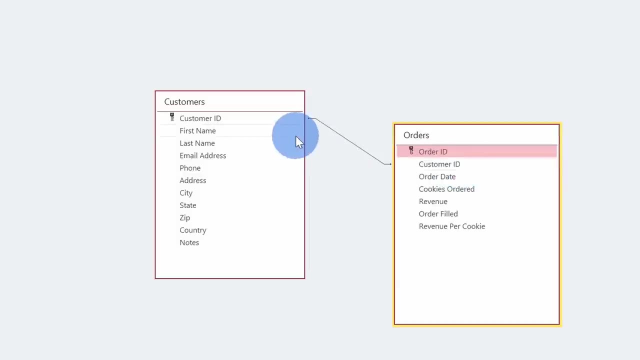 field in the orders table. So right now I'm saying that these two values or fields are the same. Next I'll click on create and you'll see now that there's a connection between these two. So this is how Access knows how these two tables relate to one another. 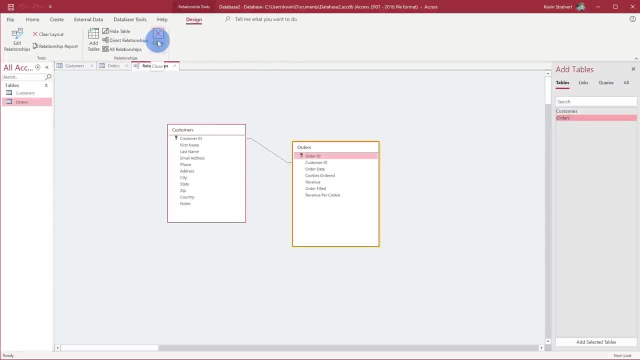 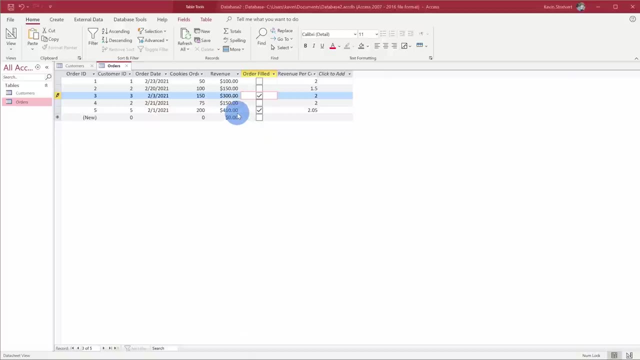 Once we're all done with this, let's go to the top and click on close. This opens up a prompt to save the relationships. I'll click on yes. Along with manually entering in data into your database, you can also import it from other sources. 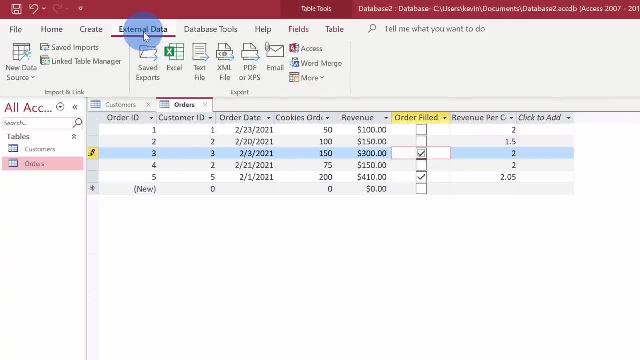 Right up here on the ribbon there's the option for external data. When we click on this over on the left hand side, you can see all the different places that you can bring data in from. For example, you can bring it in from a file, from a database, from different online services. 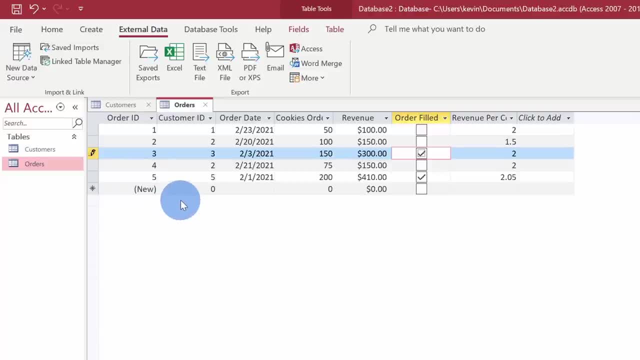 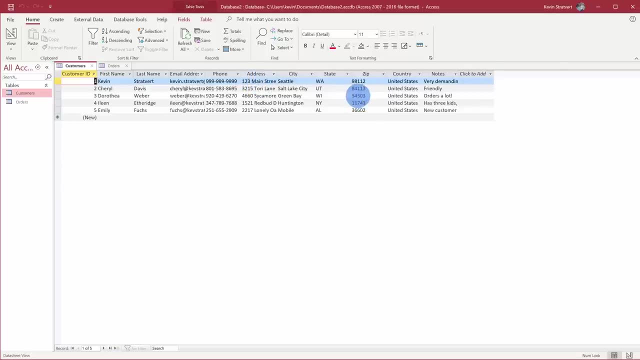 So there are lots of different ways that you can get data into Microsoft Access. So far we've been entering data directly into the table view. But let's say you want to have other people in your organization come in and add data. This might not be the most user friendly view. 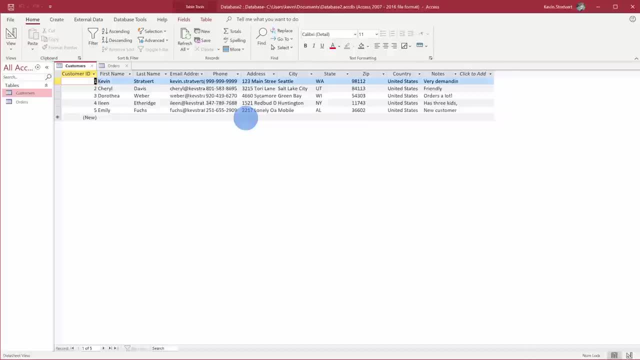 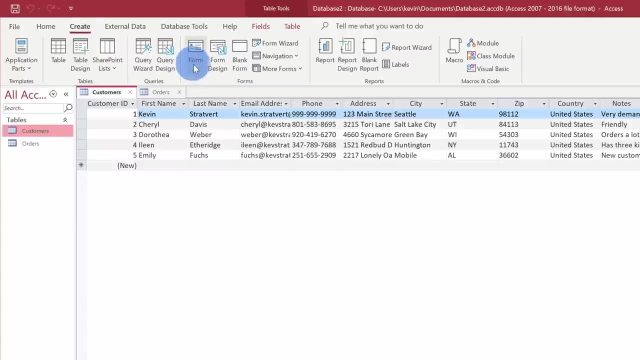 Instead, you might want to create a form that makes that easier. Over on the left hand side, I'll select the customer table Right up here. let's click on create on the ribbon And right here in the middle there is a section for forms. 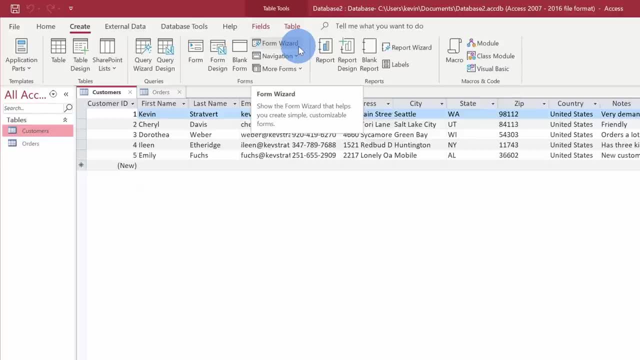 This will help us create a form for data entry, And you could also use it to review the different records that are in your tables. There's a form wizard that will help you through the process. You could also start from blank. There's a form designer or you could simply create a form. 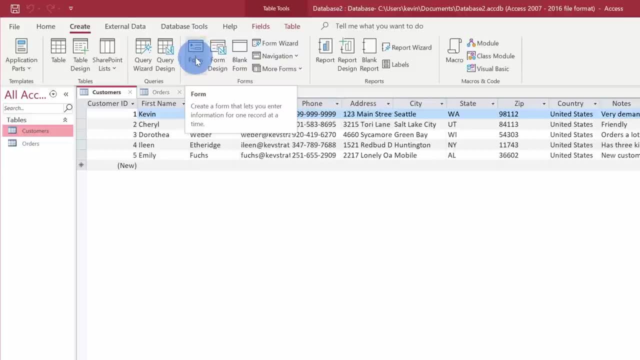 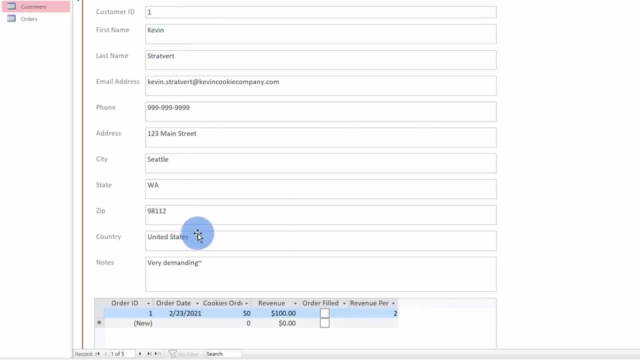 This is going to be the easiest way to create a pretty effective form, So I'll click on form right here. This now drops me into a new form, And down below I can see a sample of what the form looks like. So this will be a lot easier for others to come into and start adding information. 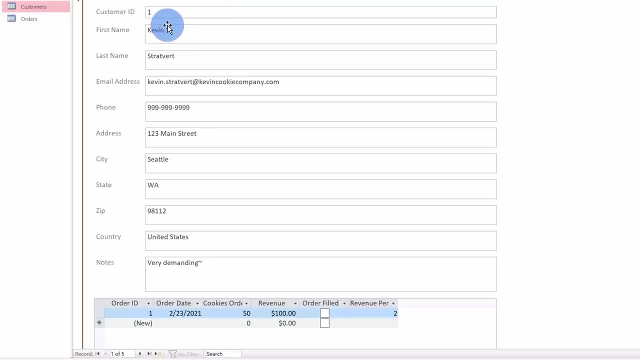 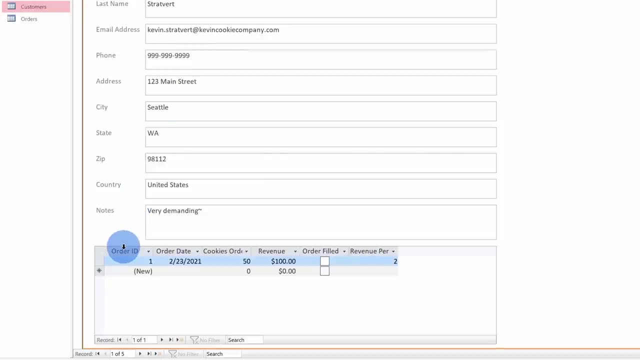 And they could also use it to review information. Now, because we connected the customer table to the orders table, you'll see here all of the customer information shows up, And down below it has all of the related order information. So here, if I jump through the different records here, I could go to the next record. 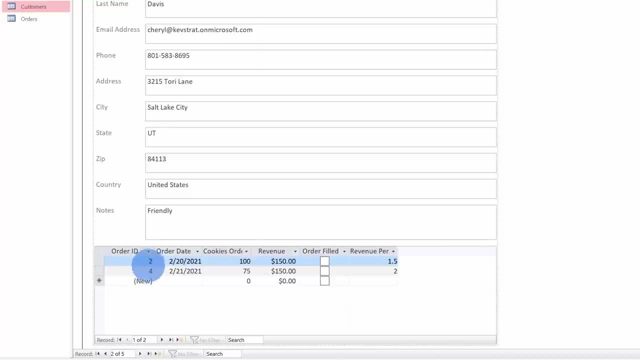 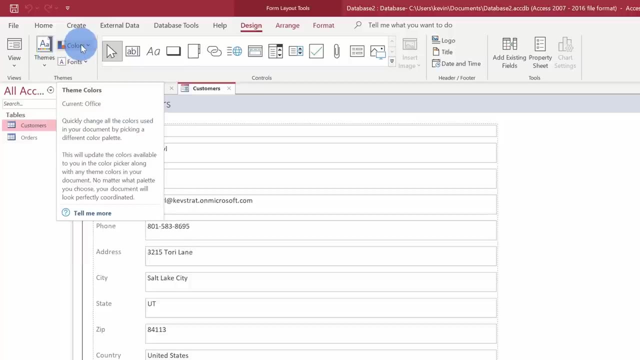 Here I see Cheryl as my second customer and she has two orders associated with her Right up on top. I can design what my form looks like, So I can choose different themes. I could choose different colors. I can add different controls to my form. 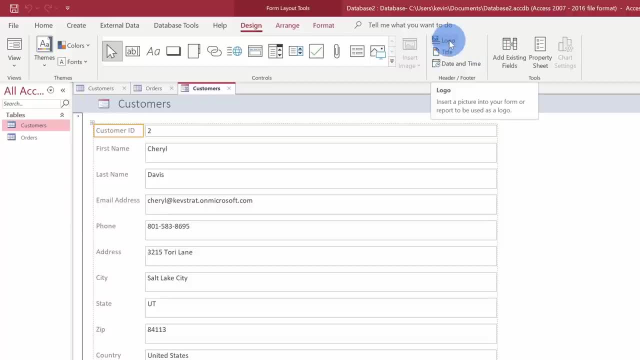 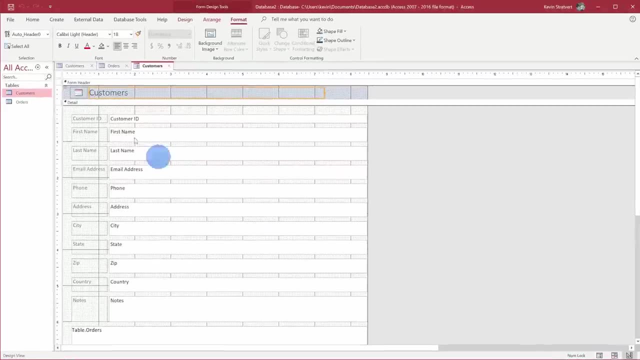 I can even add a logo, if I wanted to personalize it with the Kevin Cookie Company logo Down in the bottom right hand corner, just like we could do in the table view. here I can launch the design view And within the design view I can modify what this form looks like. 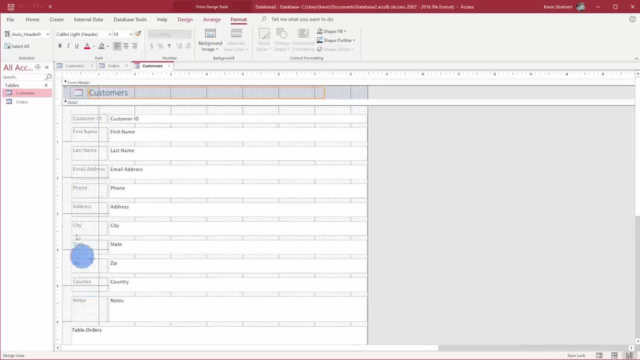 Right up here there's a form header, There are also details And here I see a footer. I can take these different elements and I can move them around. I could design the form how I want it to look. Over on the left hand side, right down here, I could also launch the form view. 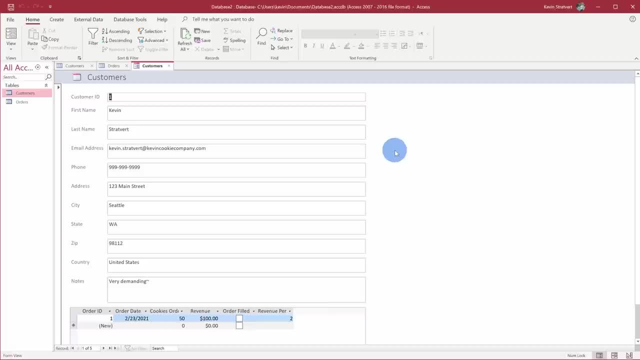 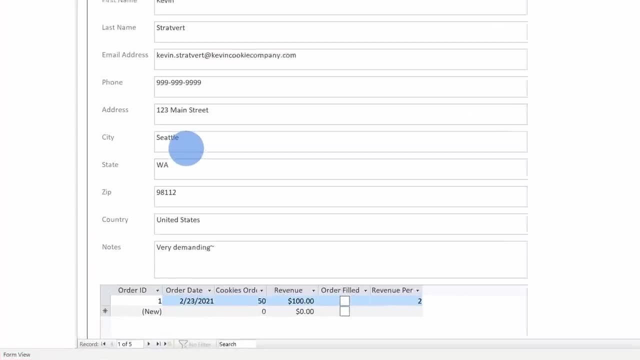 If you're going to have people in your organization going through and filling out forms, this will be likely the view that they see Here. they'll see all the customer information, but they won't be able to modify the form To add a new customer record. you simply go down to the bottom and you can click on this icon to add a new blank record. 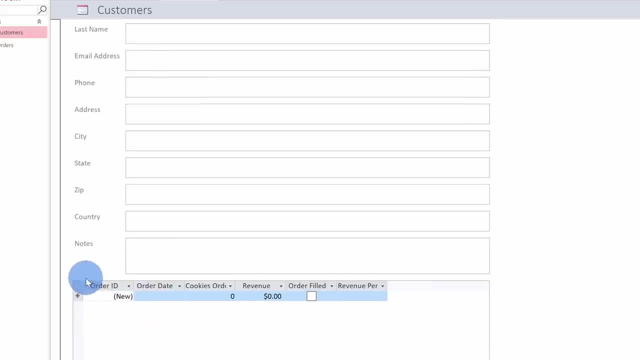 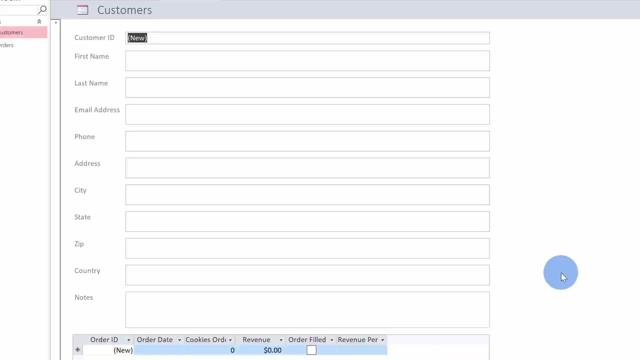 When you click on that. you can then go through and you can fill out the form And right down here someone could go in and add some additional order ideas. So this makes it really easy to get new data into your database without having to see the tables and all of the details of the database. 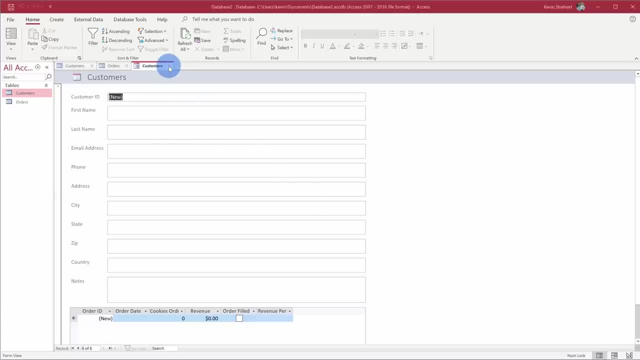 Once you're all done customizing your form, we can close out this form. Right up here, let's click on the X icon and I want to save this form, So I'll click on yes and then you can give it a name. 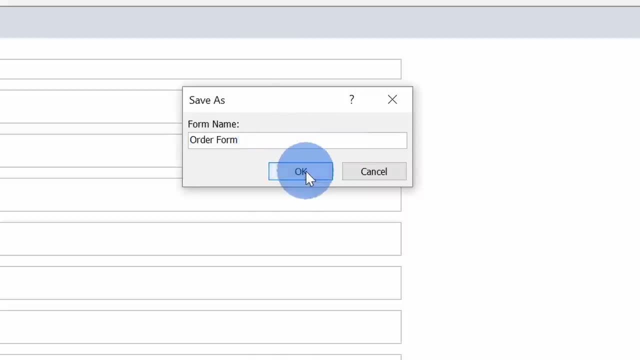 I'll call this order form. Once you're done typing in the name, click on OK Over on the left hand side. now you'll see that it added a new category. So we have our tables and now we have a new form. 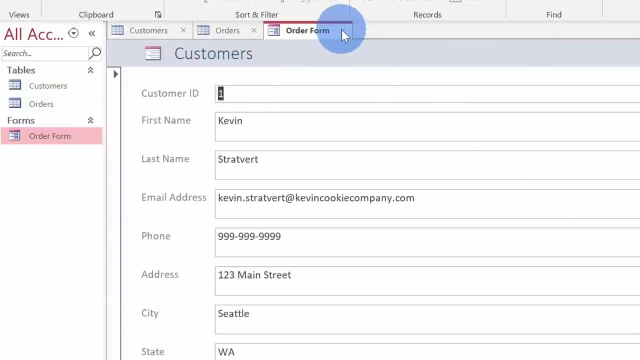 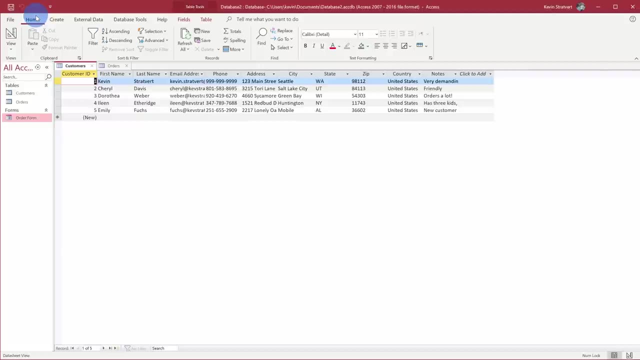 I can double click on order Form and this will open up that form again. in the introduction I mentioned that much of the power of databases comes from being able to run queries, And in a moment I'll show you how you can run and also write your very own query. to create a query. 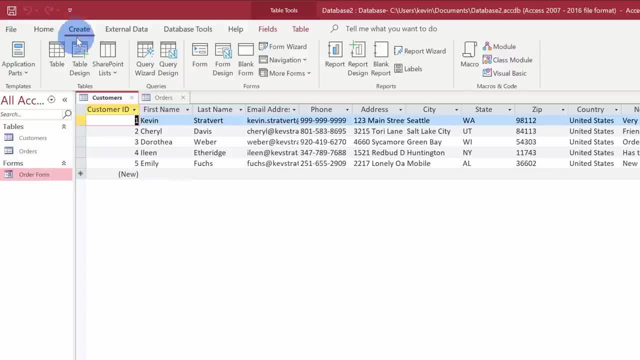 Let's go up to the top ribbon and click on create within create. right here near the middle. There are two different options for queries. You can use the query wizard and there's also something called query design. We're going to use query design. 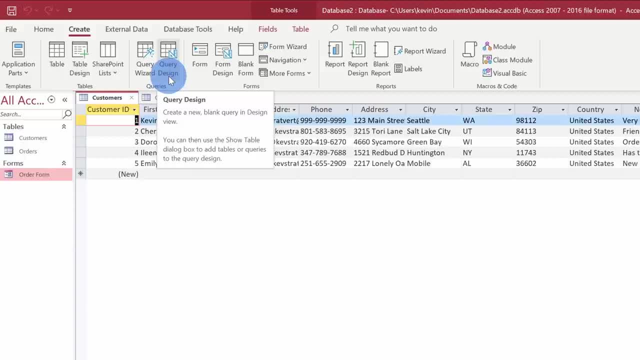 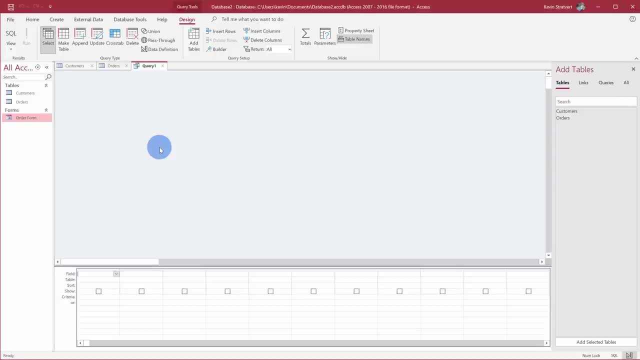 You'd be amazed at how many advanced queries I've written using query design. Let's click into this. This opens up the query designer and I want to write a pretty basic query that shows me all of the orders that haven't been filled yet. 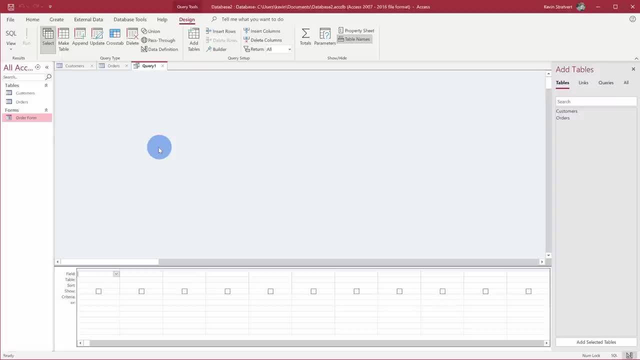 I need to provide this to the warehouse crew so they can send out the orders Now, right here in the designer. right now, we just have a blank slate. How do we start building out a query? And once again, this is just a drag and drop way of building queries. 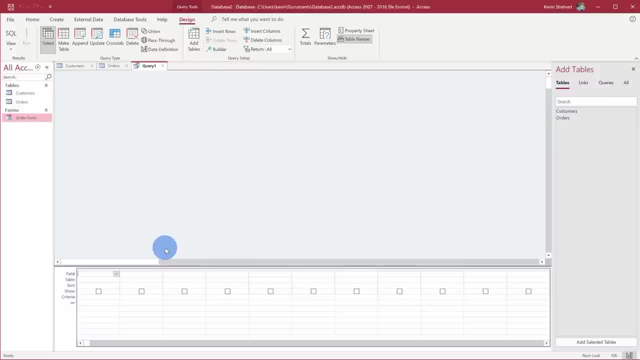 So it's extremely easy. In a moment I'll show you what the SQL looks like to actually run the query. but we're just going to start out with this GUI or this graphical user interface. first, Over on the right hand side, you see this pane that's called add tables and we want to query against the data that's in these tables. 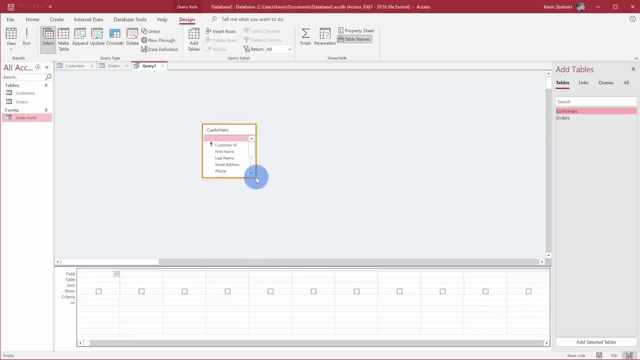 So I'll take customers first and I'll drag it out into this view Here. I'll expand the rectangle just so we can see all of the details Right next to it. I also have orders. Let's click on that and let's pull that in as well. 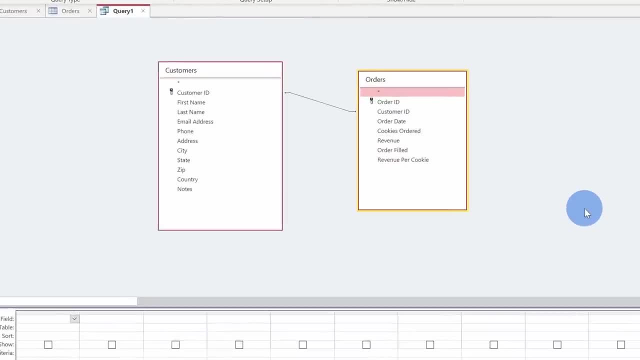 Here I'll also adjust the size of this rectangle. In an earlier step we went through and we defined a relationship between this customer ID and this customer ID, So these two tables are connected. So I could do things like for a specific customer: show me all of the orders, because these two tables are related. 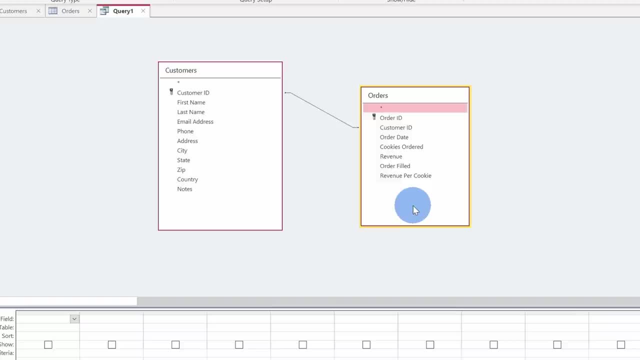 Now, once again, I want to show all orders that haven't yet been filled, And for this I'm going to send it to the warehouse crew, And so they're going to need stuff like: well, what is the customer's name and what is their address where they should send the order? 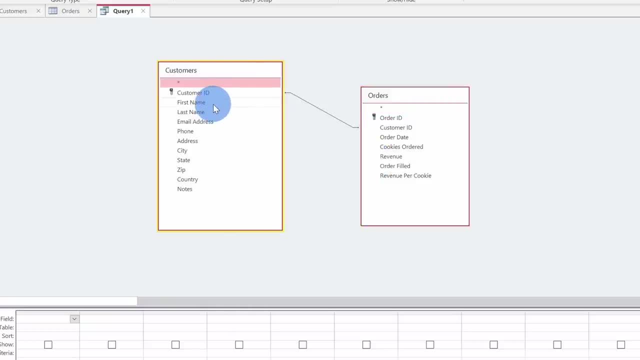 So over here I want to pull in some information for this. So I'm going to pull in some information for this. So I'm going to pull in some information for this query. I want to show the first name, So I'll double click on first name. 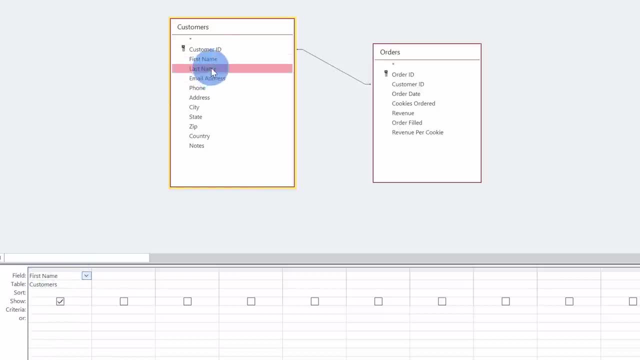 Here you see that first name shows up down below. I also want the last name. I want the customer's address, the city, the state and also the zip and the country. They're going to need all of this information to send cookies to this customer. 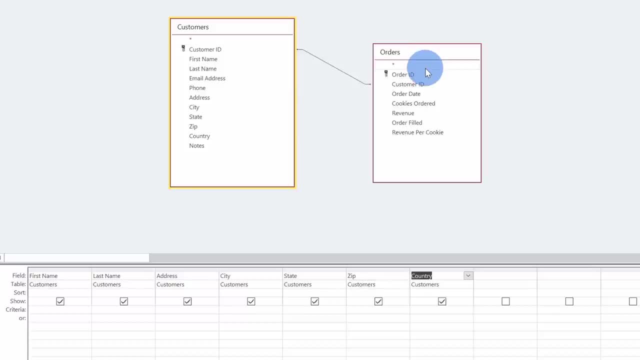 Now, over on the right hand side, I have some additional information and the warehouse crew is going to have to know. well, what was the order date. They also need to know how many cookies were ordered, but they don't need to know stuff like the customer ID or the order ID. 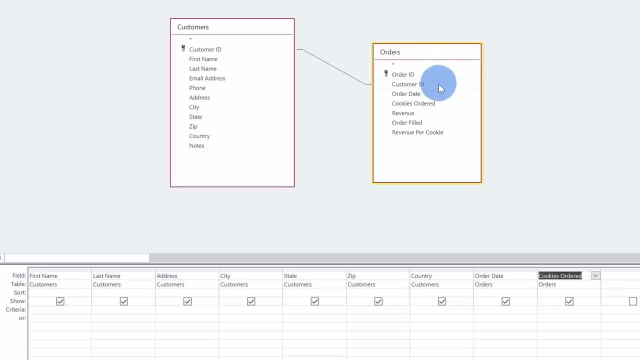 That's not really essential For what they're doing, So I won't select these right down here. There's also the option that says order filled. Let's click on that one Now. this is all going to run a query, and it'll give me back all of this information. 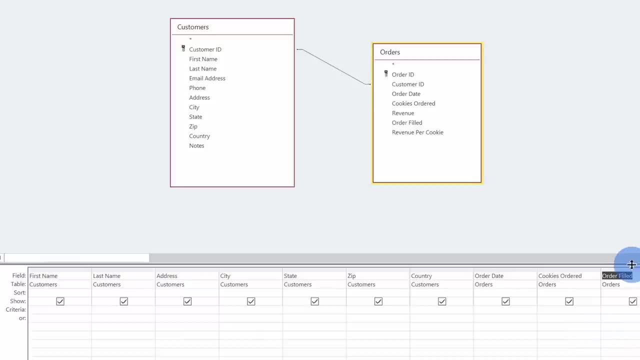 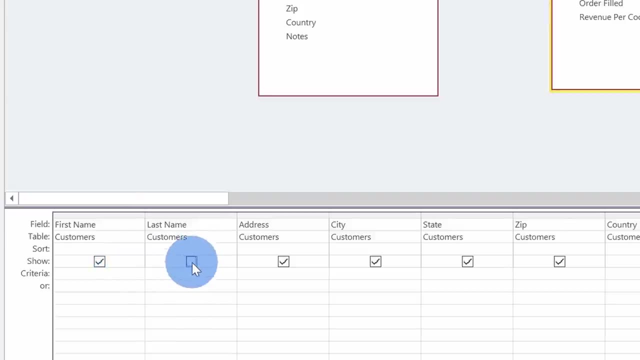 But once again, I only want to show the orders that haven't yet been filled. You'll see down here. it shows the field, It shows the table. it's coming from here. I could sort it. I could also decide whether I want to show it or if I don't want to show it. 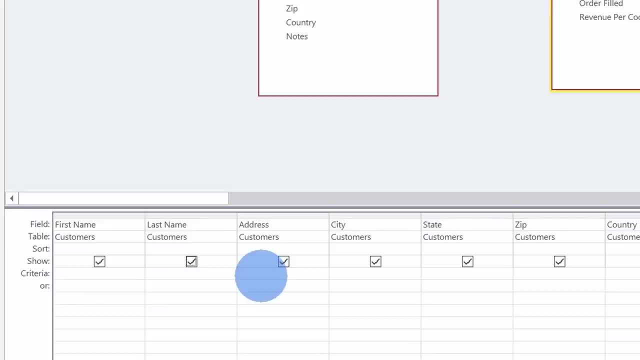 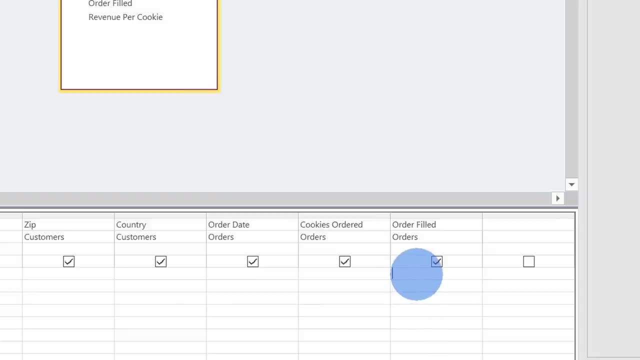 And right down here I can define criteria. So this is kind of like, or basically it's a filter. for one of these These fields over on the far right hand side I see order filled and for this one I'm going to enter an equal sign and then type in no. 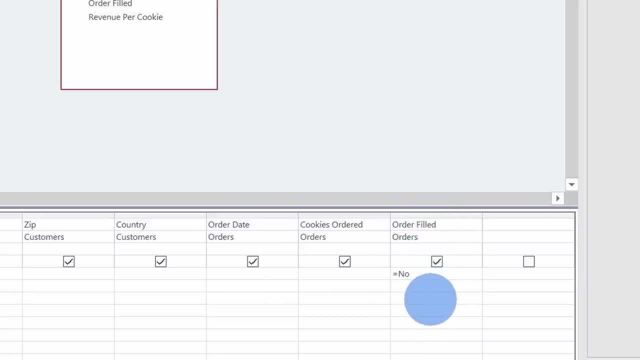 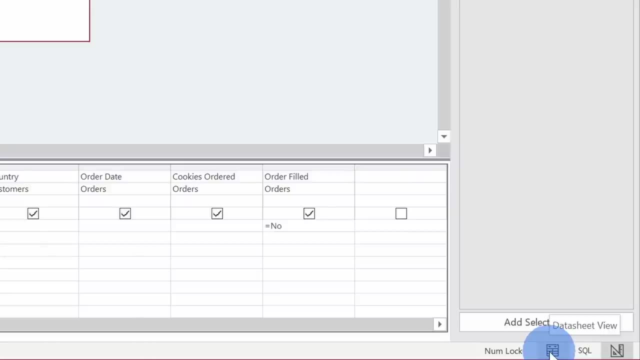 So this means that the order hasn't been filled yet. So right now I have my query in place. down in the bottom right hand corner I can click on the data sheet view. Let's click on this to see what the results are When I click into the data sheet view. look at that. 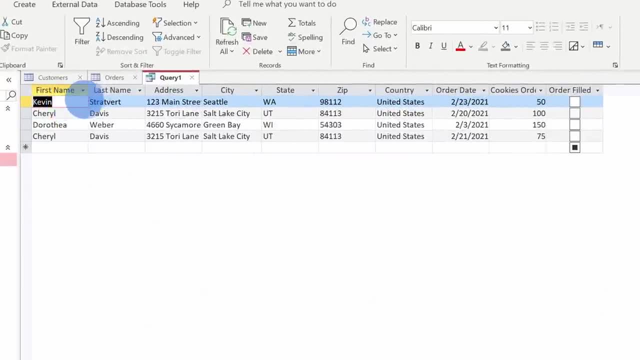 That's our first query. So here it returns all of the different fields that I selected, and it also only returns all of the options where the order hasn't been filled yet. Now one of the really neat things is here. now I'm merging together customer information. 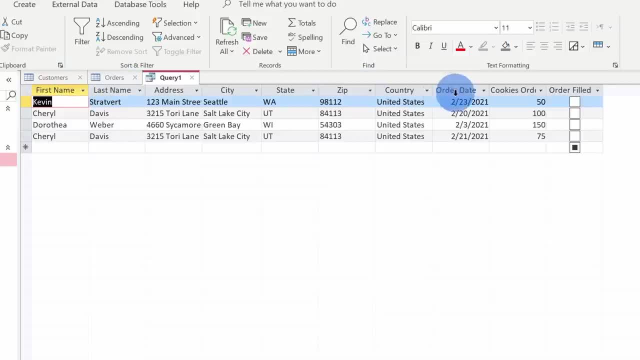 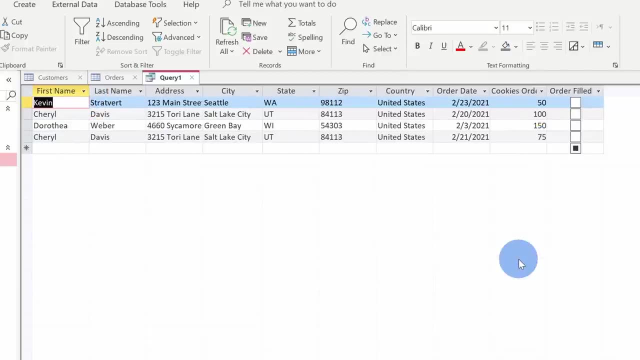 So data from the customers table together with data from the orders table, So it brings it all together in one view And that's what I can pull off using a query. Now, so far, we just used a graphical user interface to pull off this query, and it's pretty impressive what you can do. 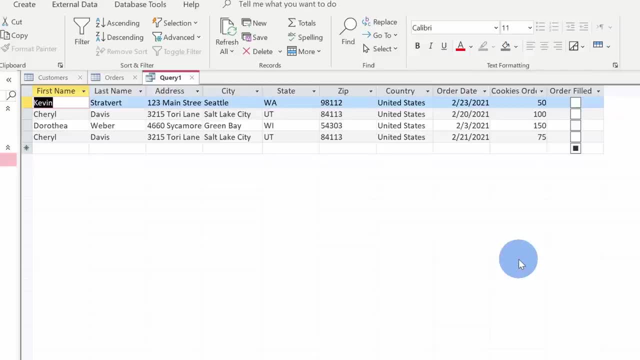 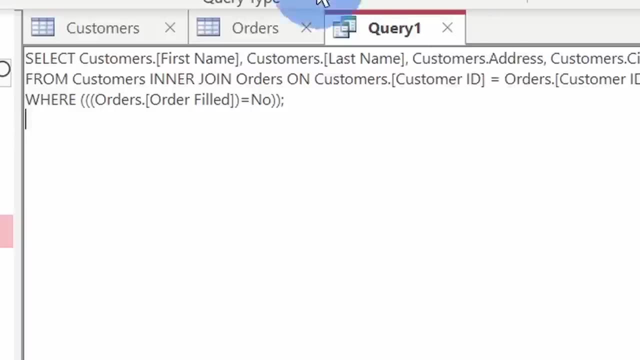 But you might want to get your hands dirty and write a SQL query Down. in the bottom right hand corner we can see the SQL query That powered this. When I click on SQL right here, I can see the actual SQL query. So right up here we're selecting all of these different fields. 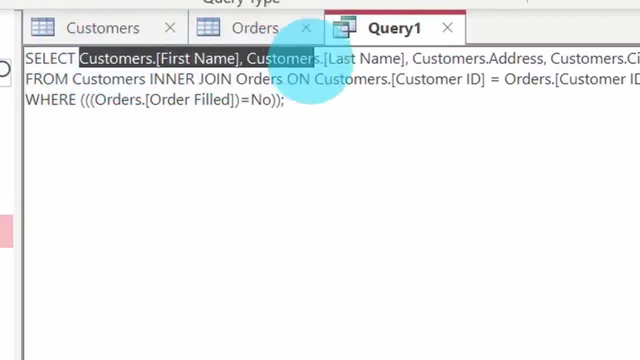 We use a select statement and then we call out: well, hey, I want the first name, I want the last name. And we go through and we identify all of the different fields that we want. Then next we're saying where it's coming from. 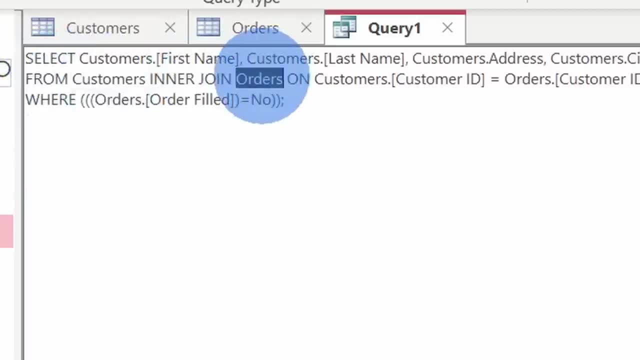 So we're pulling it from the customers table and then we're going to join that with the orders table And we're making that connection on the customer ID And then down below this is where we have our customer ID. So we're saying where order and orders filled equals no. 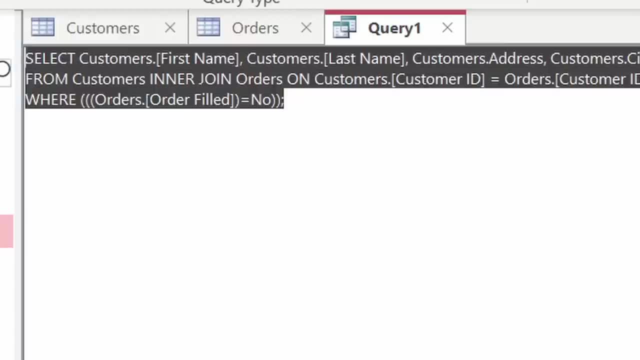 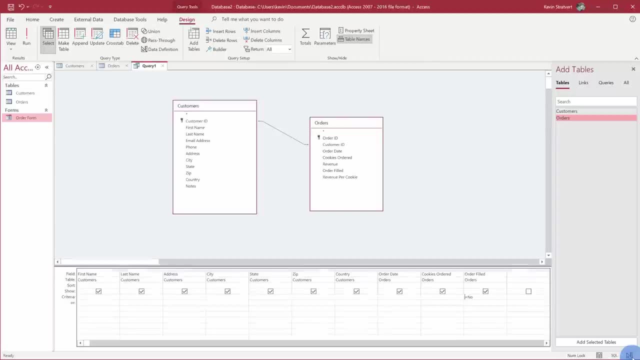 So this is the actual SQL query. So if you want to get your hands dirty, and especially as you want to start running some more advanced queries, you can start experimenting with this. Now. the really neat thing is, you can use this designer to pull together some really impressive queries. 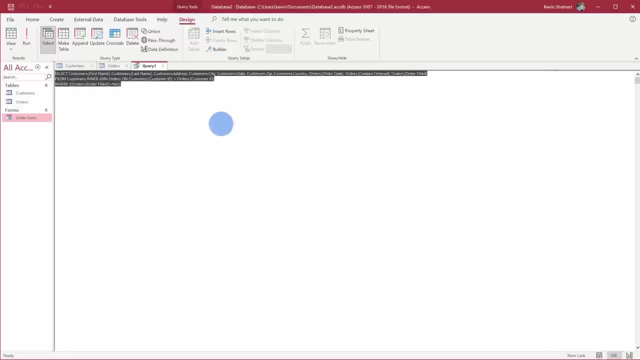 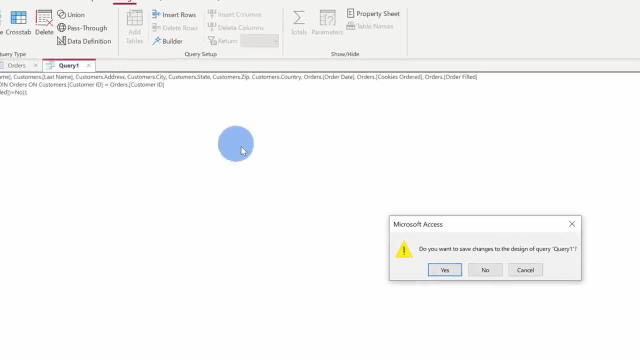 And then, if you want to see how it works behind the scenes, you can click into SQL and you can see what the actual query is. Now that we finished entering in our query, let's go up here And let's close out This view, and I want to save this query. 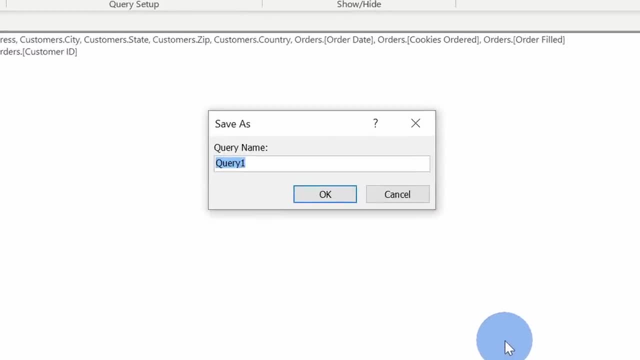 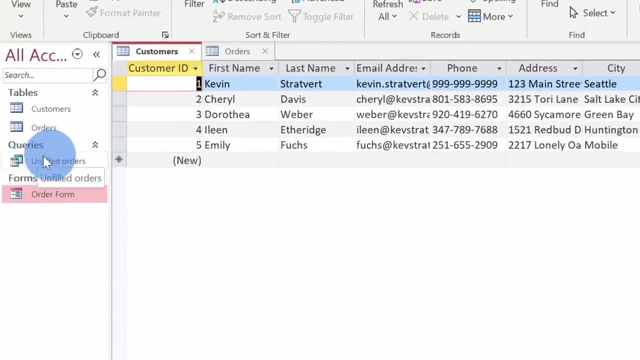 So I'll click on yes and we're going to call this unfilled orders. Once you're done typing in the name, click on OK. Over on the left hand side you'll see a new category now for queries and this shows our unfilled orders. 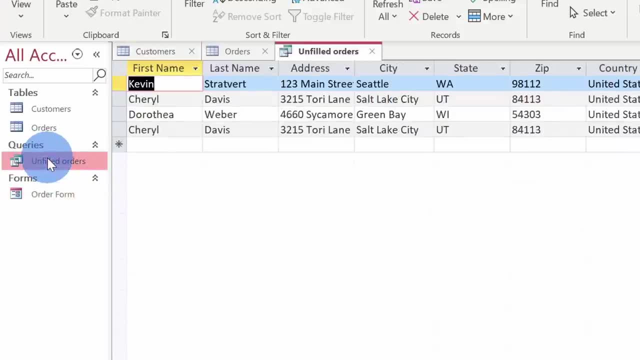 So if you want to quickly see all unfilled orders again, you can simply double click on that And right now I have a view of all of the unfilled orders. Now the really neat thing is, as you go in and you add, let's say, additional customers and additional orders, if you have any unfilled orders and you run your query. 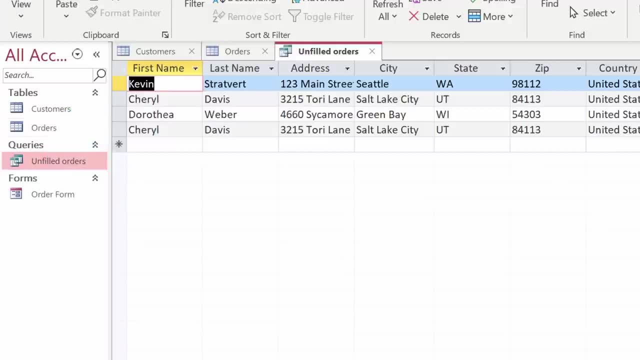 You'll immediately see them on this page. So let's say, I have warehouse staff and they always need to know what orders have we not finished yet. They can simply run this query and they'll immediately see all the orders that need their attention. So it's pretty powerful stuff. 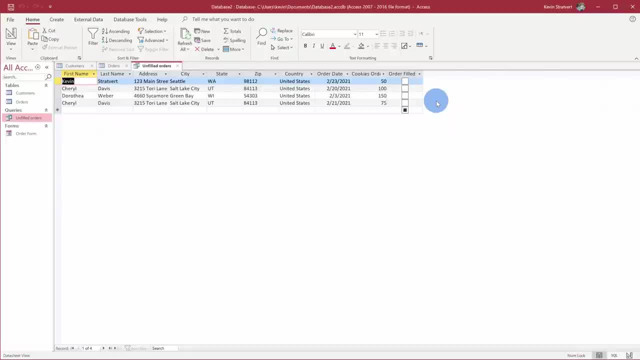 Lastly, I want to show you how you can create a report. So let's say that maybe management or someone else in the organization needs to see a summary of data, Or maybe for the warehouse crew, instead of having them come into this access database and run the query, maybe every morning, I want to print out a sheet of all of the orders. 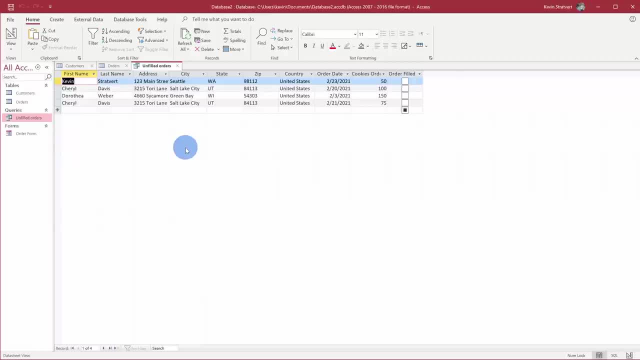 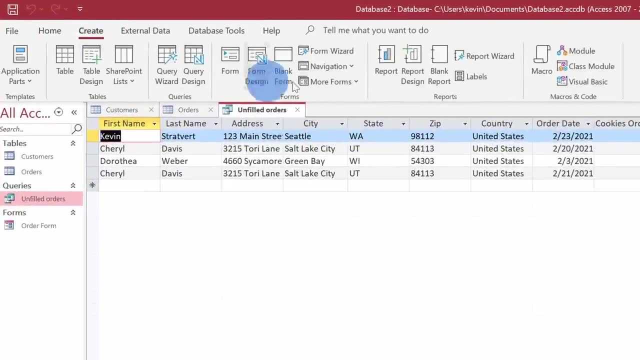 That they have to fulfill, and I can use a report to do that. to create a report, just like we created a query, Let's go to the top ribbon and click on create. over on the right hand side There's a section for reports and we can click right here to create a report, and there are a few different options. 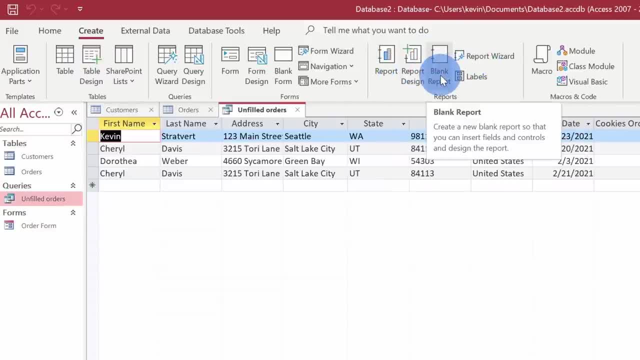 You could use a report wizard, You could use a report designer, You could even start with a blank report. So depending on how much you want to customize it, you have different options here. Now I want to create a report that shows all of the unfilled orders. 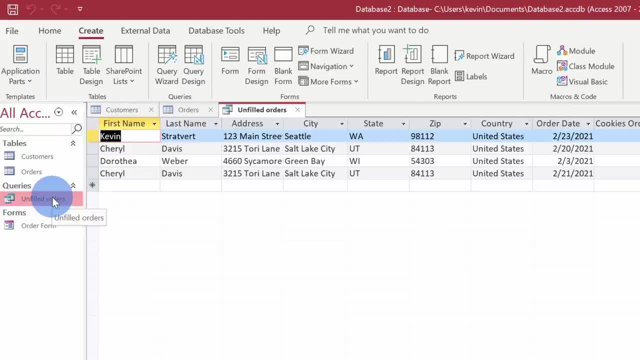 So I'll make a report. I'll make a report, I'll make a report. I'll make sure to select this query over on the left hand side. If, say, you wanted to create a report of all of your customers or all of your orders, you can select those tables and then click on report and that'll create a report of those items. 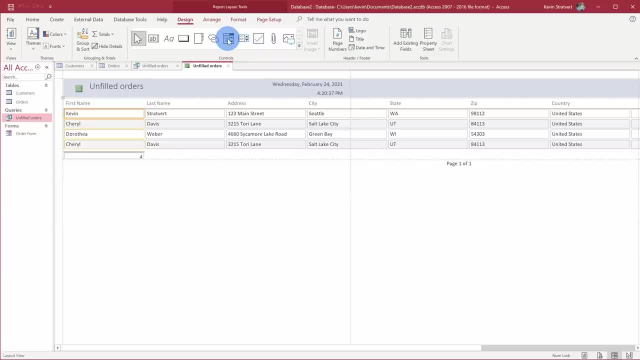 Here, with unfilled order selected, I'll click on report. This now generates a report with all of the unfilled orders. So here I see all of the information that I selected in the query, and it's all formatted in a very nice way. 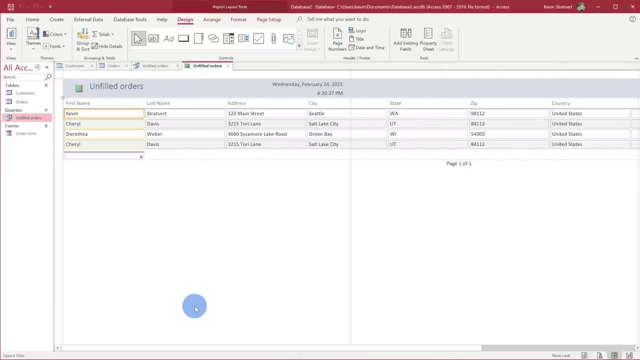 And here I can go over and I can see all of the details Right up here. I can format the report however I want. I could go, I could go through, I could choose themes, I could choose colors, fonts. Even down here I can preview what it'll look like when I print it out. 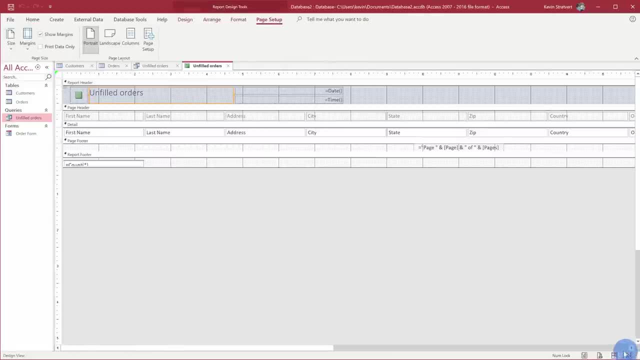 Here I can see a report view and here I can access the report designer So I could go through and design specifically how I want this report to look. So I have quite a bit of customization. Once you're all done configuring your report, you can close it out and then you can save this report.